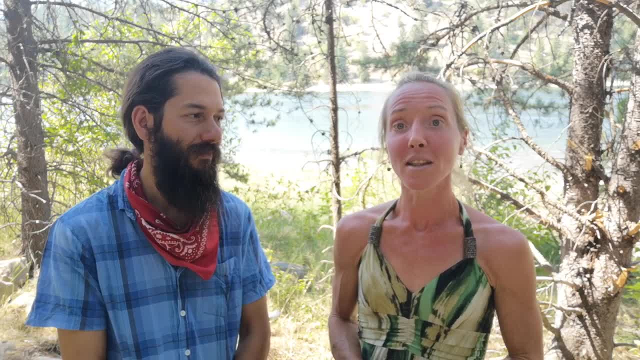 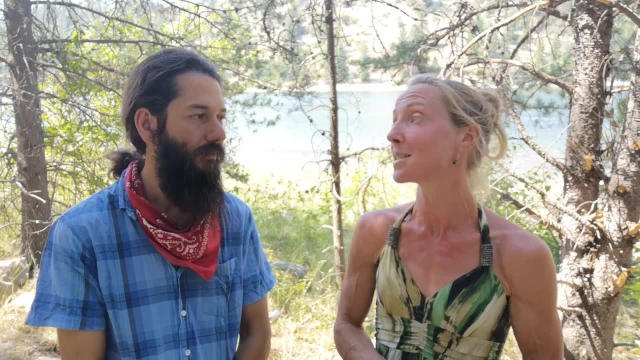 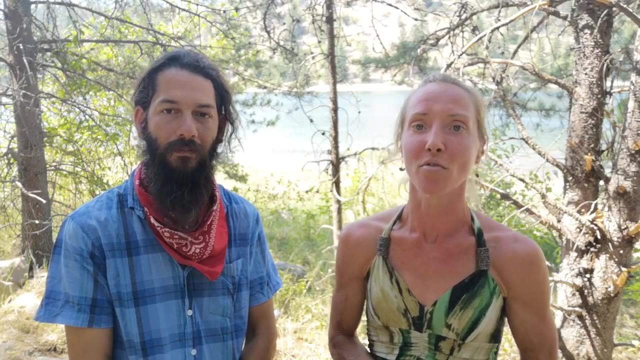 friend in Kamloops, Kent Watson, who was willing to interpret some of the data that we received back from him, So we were hoping that he could break it down a bit more for us. Well, thank you. Yeah, thank you so much for meeting with us. We have been scratching our head trying. 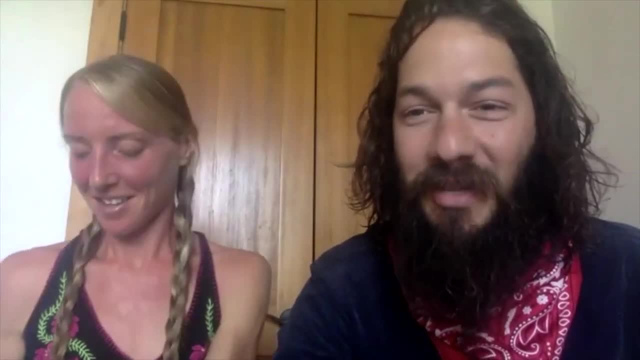 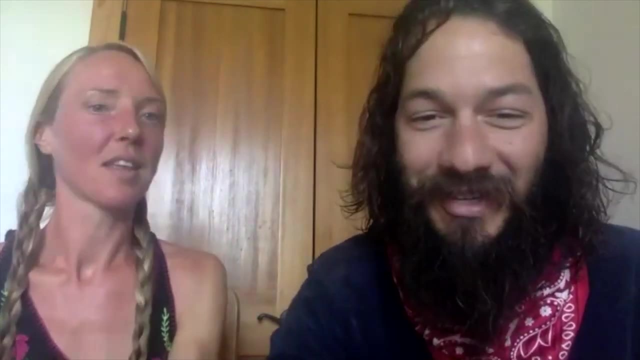 to figure out a way like to understand the test results and, without you know, perfect opportunity. we'll contact you and see what you think about it. Okay, so before I get into the question, do you want to just give us a little bit of background on what you've been doing in the past? 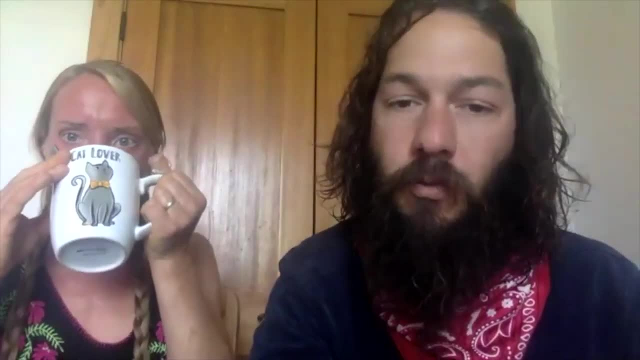 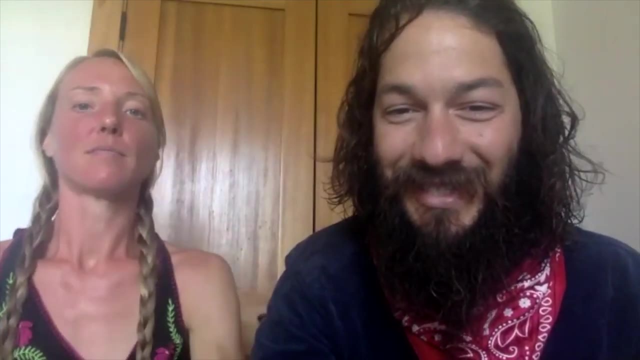 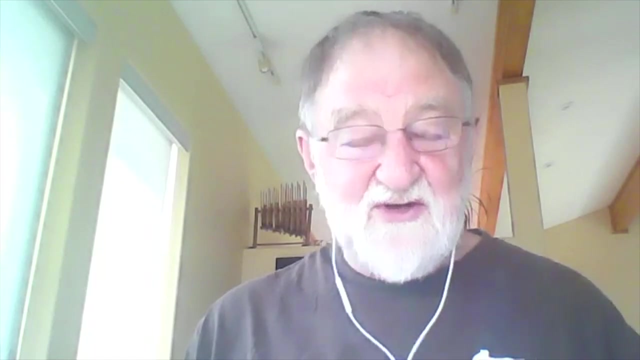 Sure, Do you want to just give us a little bit about your own background or how you got into soil science so that we can share that with people before we start talking about the questions? Sure, I did my master's degree in agriculture and specialized in soils, and my main focus is 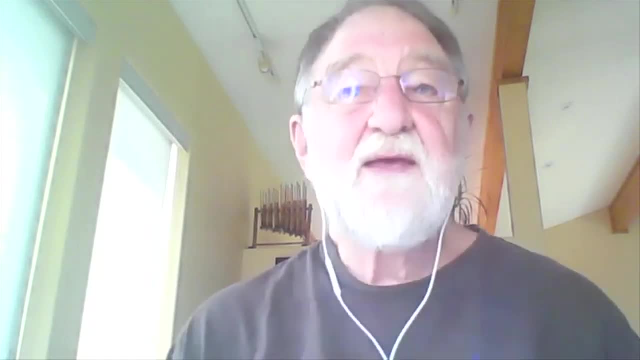 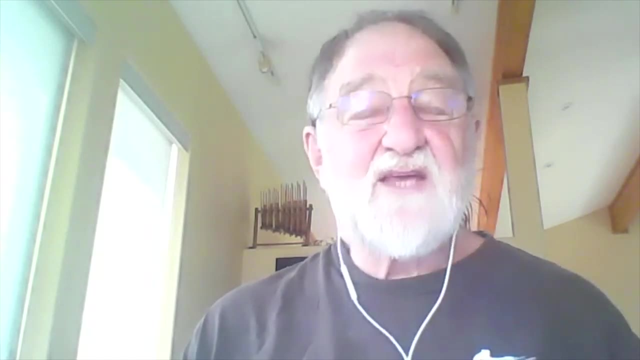 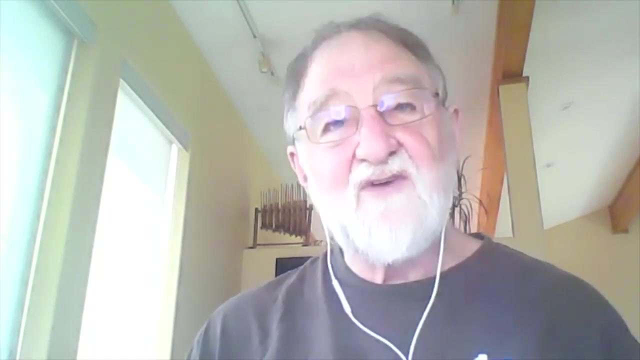 on soil classification and describing soils in the field, and that's what I do. I then got a job at was then Caribou College back in 1986 or something, when they started their forestry transfer program that developed into their natural resource science degree program, which Anastasia took. 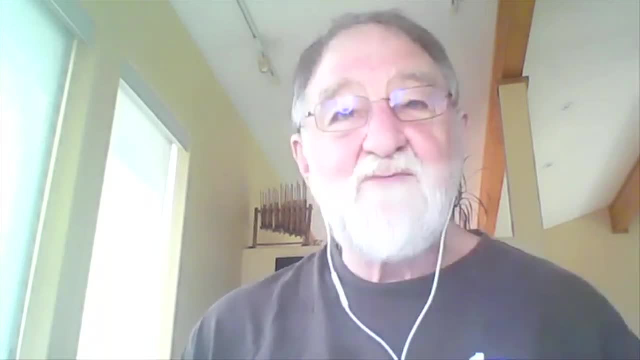 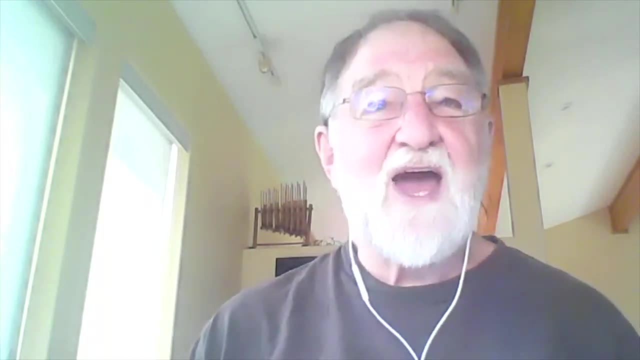 and I taught soils in there and I've just been passionate about it. I don't know why. well, I actually figured that out. I was in a soil pit one day and describing the soils for a guy, and he looked at me. he says: every time you're in the soil pit, there's this incredible smile on your face. so 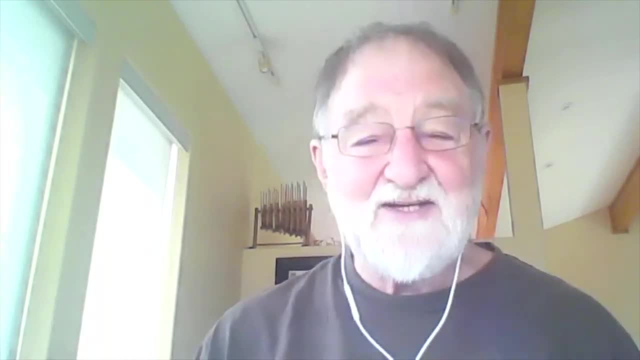 it's reconnecting to the earth? I think, I don't know, but yeah, I just, I just love it and I retired from Thompson Rivers University in 2016, but I still do soil contract work. I'm working with the Alberta Sewage Association training people who put in septic systems how to classify their soils. 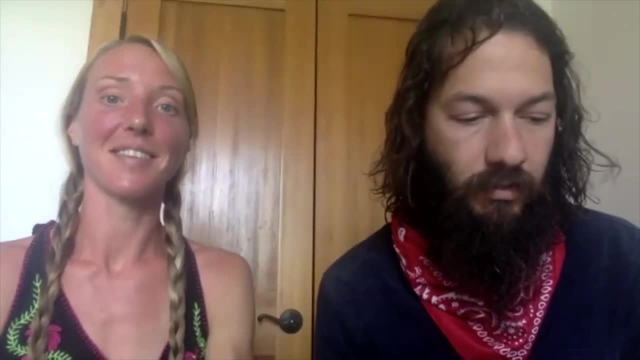 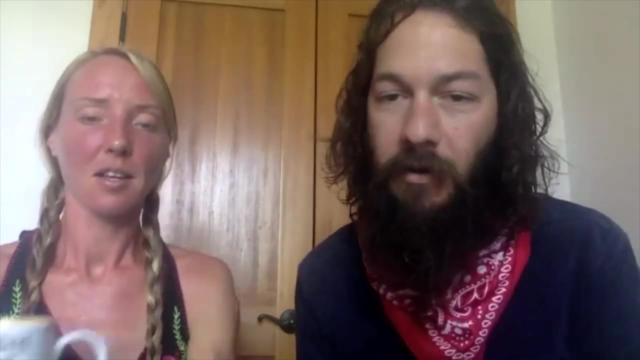 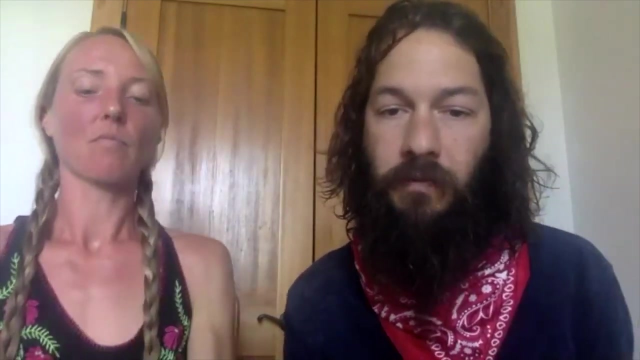 so that's my new career. Oh yeah, that's awesome, awesome and okay. so the first question we have is: basically, we got you know we were concerned about heavy metal contamination because of the history of the land that we're really seeing, so there was back in the day, the coming code was: 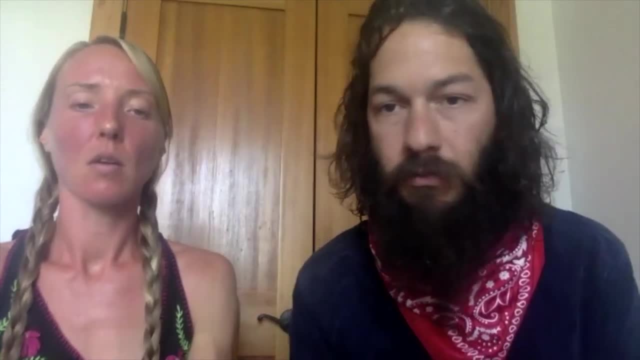 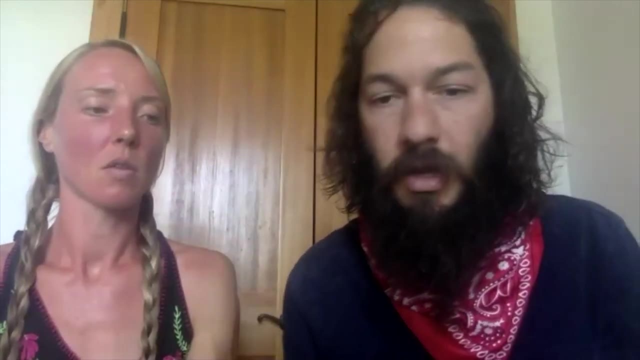 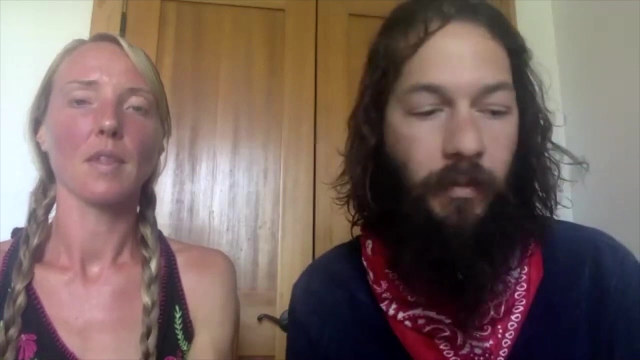 polluting the whole area around trail and calciger and much larger area, and so there's evidence that some places still have heavy metal contamination in the soil. so, to be safe, we decided to do a test as well, so we shared the full test results with you. but how do we go? 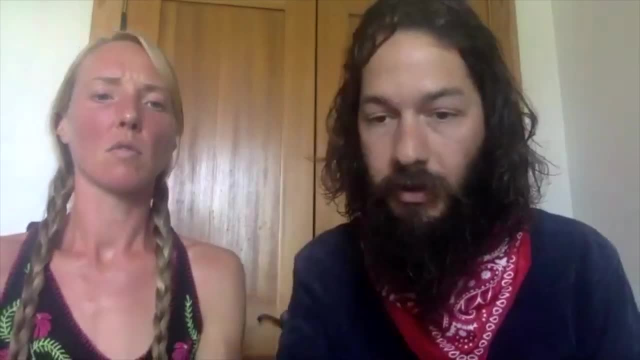 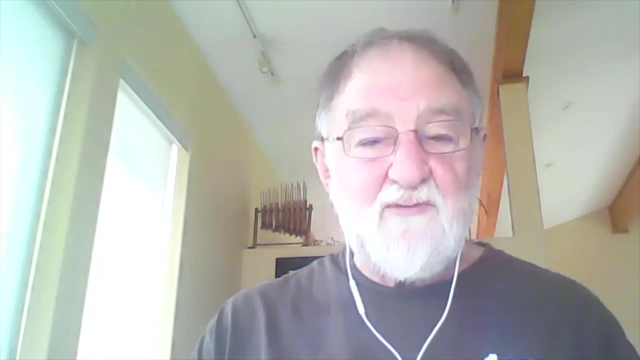 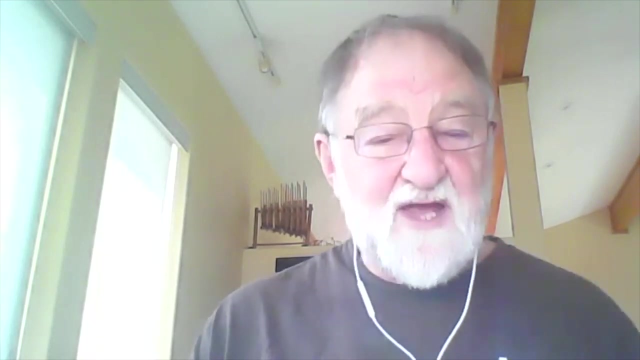 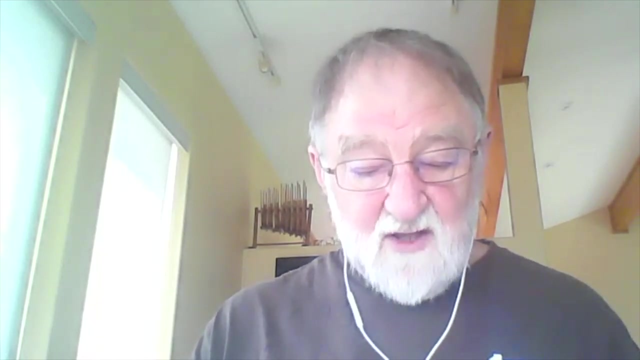 How do we go about interpreting that result? Well, first of all, I have some tables here from another report. I've been reviewing soils data and reports from Highland Valley who are planning to expand their mine, so I pulled out these tables and they're from the Canadian Environmental Quality Guidelines. so if you type in CCME guidelines, it'll tell you the results. 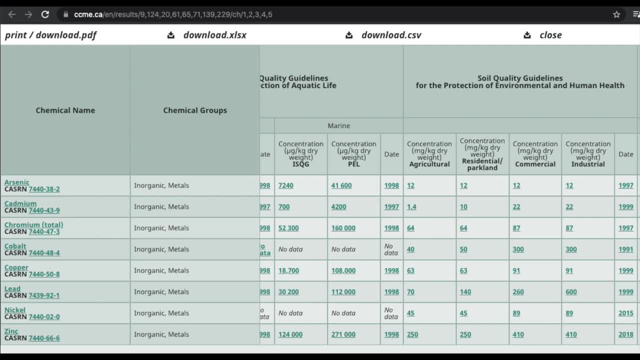 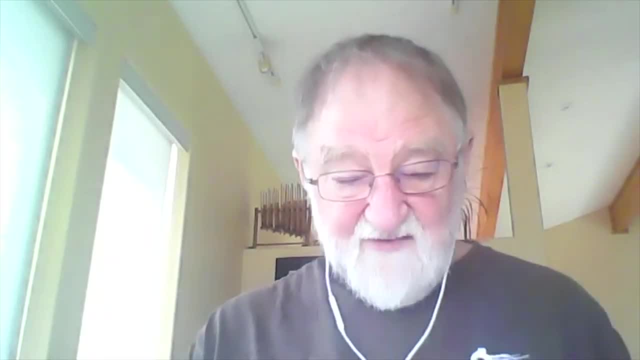 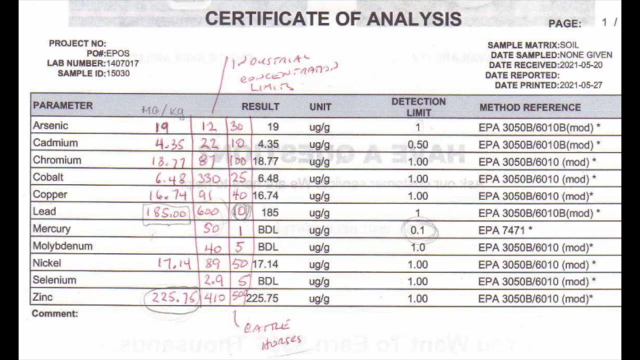 They'll take you to that site. Once you're there, you have choices as to where to go, but what I have is tables of the heavy metals from the report I worked on and the industrial concentrations and the maximum tolerance levels for cattle and horses. okay, right, so what I did is I went through that table and, with your data, that you sent. the only thing that is over one of the guidelines is the industrial concentration limit for arsenic. it's 19 milligrams per kilogram and the industrial concentration limit is 12, but the cattle horse consumption can be up to 30. All of your other results are less than these standards. 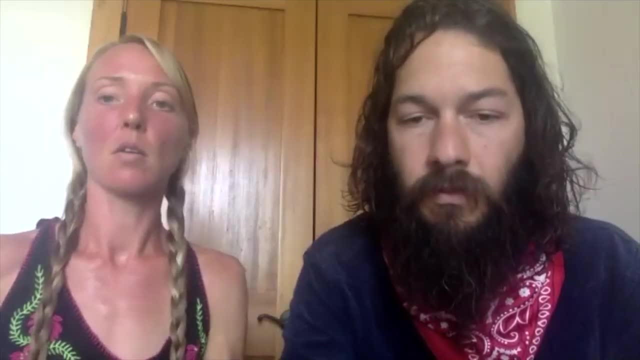 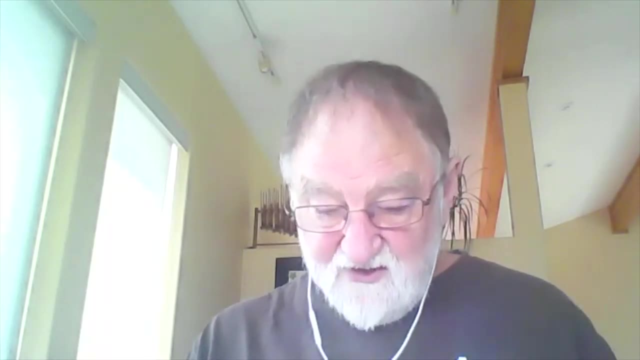 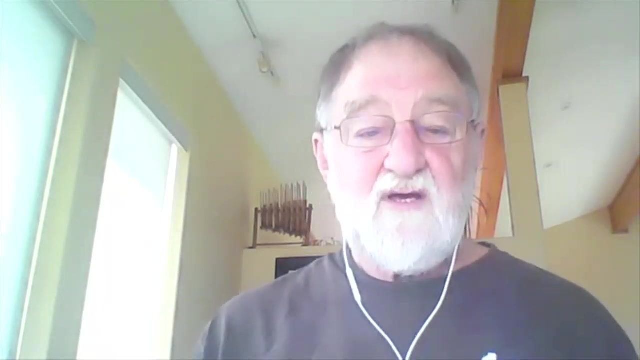 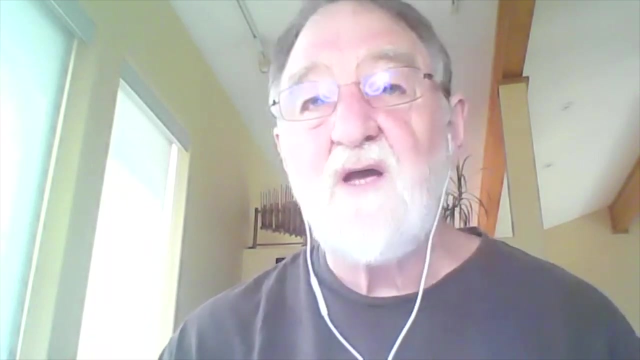 Okay, They're all less and um in most cases like they're like considerably less, so these results look good. I wasn't aware that Kaminko was in that part of the world, but I know it did a lot of pollution damage and I remember going through trail many, many years ago when 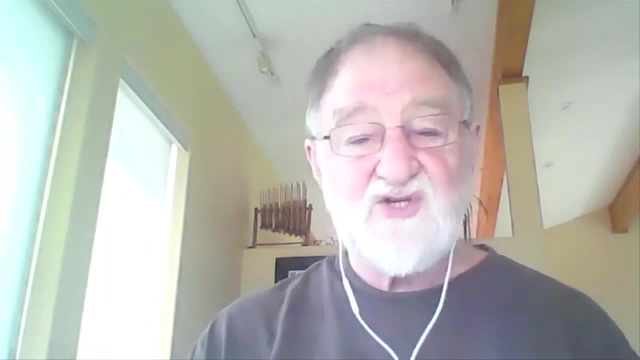 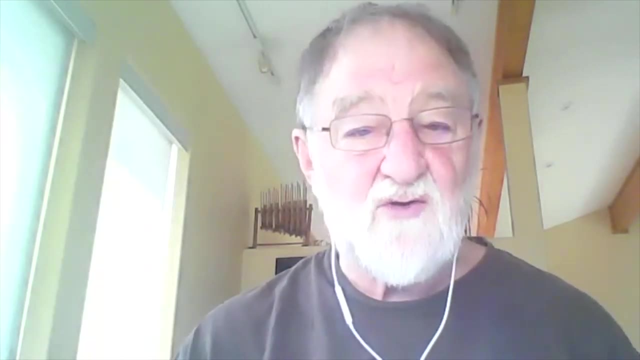 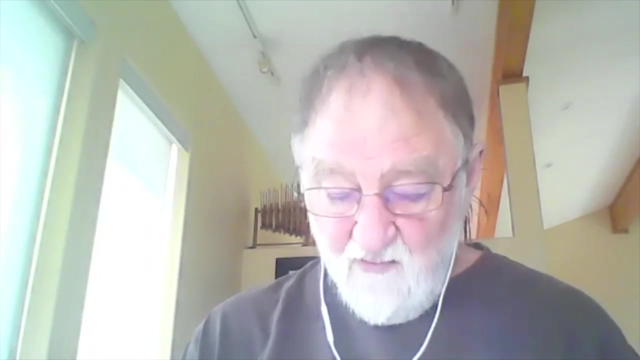 they were still operating their smelter. there was no vegetation anywhere, nothing. And now I went through trail- oh, four or five years ago on a soils tour and the vegetation has come back extremely well. So from what you've sent me, everything seems to be okay. 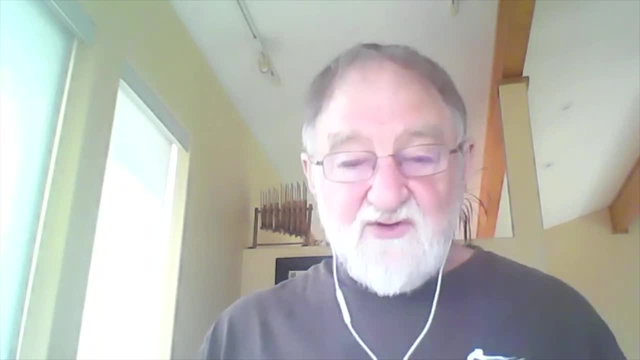 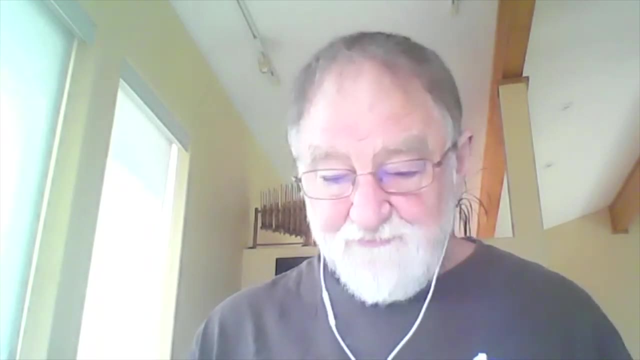 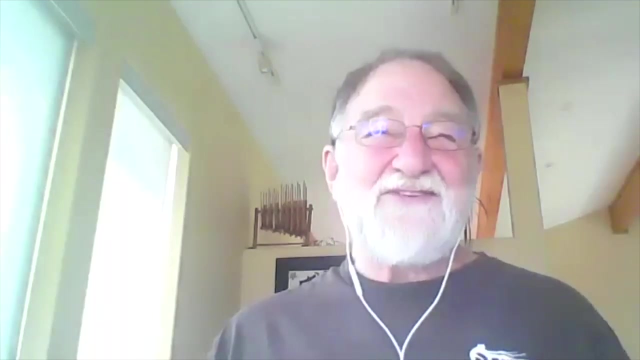 So that's from basing on this, but you could also go on to the website and if you wanted to dig for more information, you could. It means some scientific reading, Anastasia, So if you want to do that, be my guest. 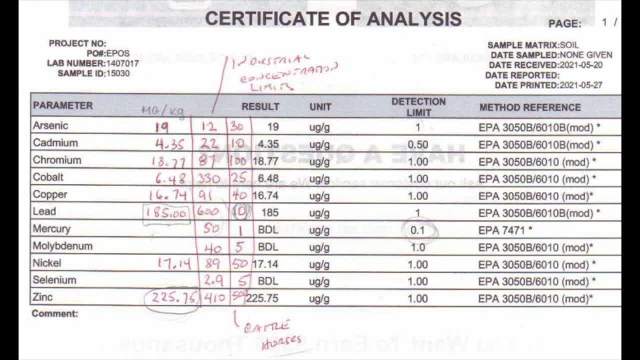 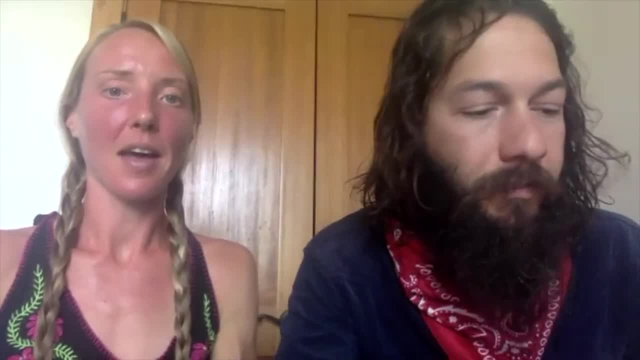 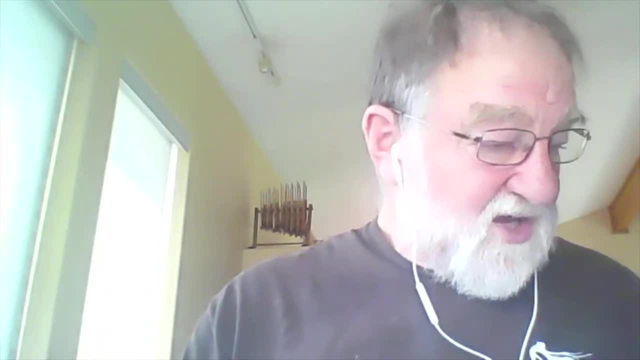 But right now, from what I'm seeing on your certificate of analysis, everything's good, Awesome, Okay. Yeah, That helps a lot. Yeah, that's very encouraging. Yeah, thank you. I have also a table here That I can scan and send you as well. 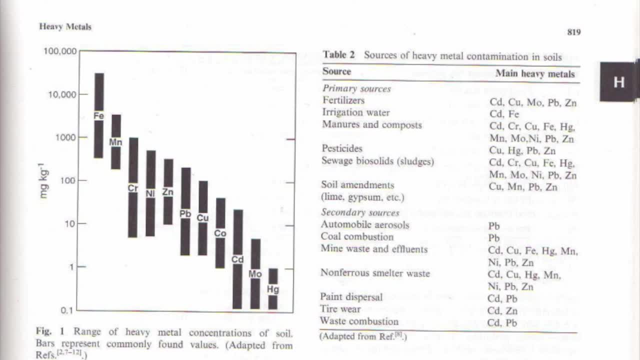 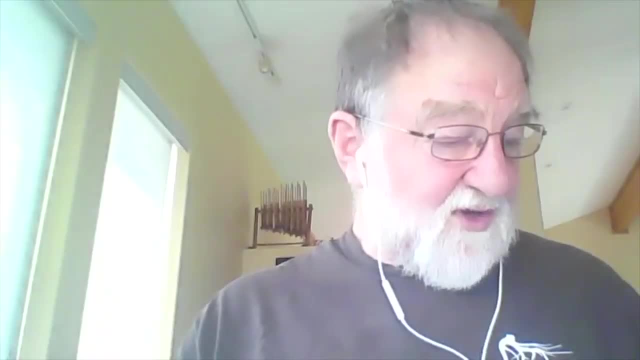 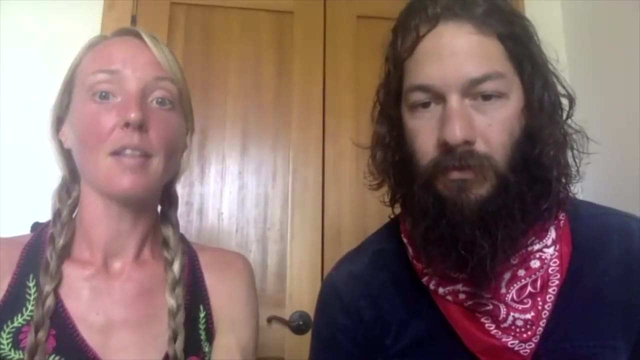 That gives the range of heavy metal concentrations in- Actually I can scan the whole article for you- Heavy metal concentrations of soil in soils and it gives the range of all the heavy metals that naturally occur in the soils And I think that will be helpful for you to see. 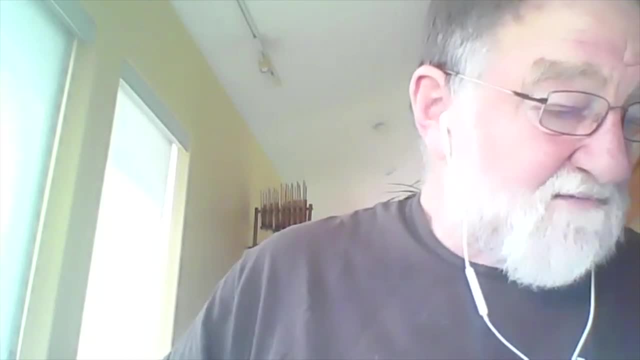 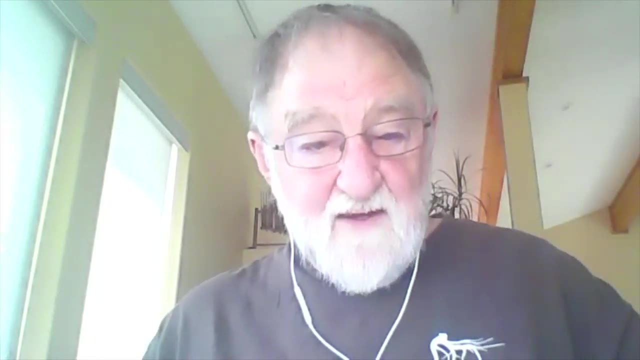 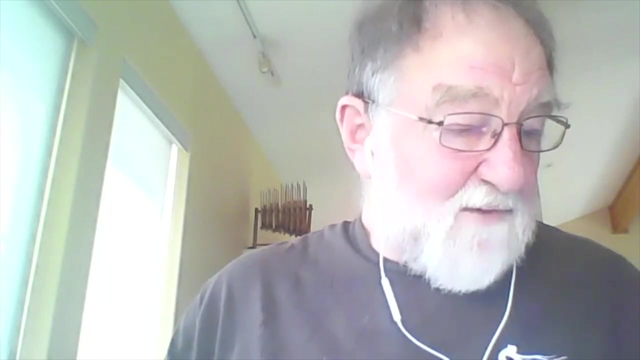 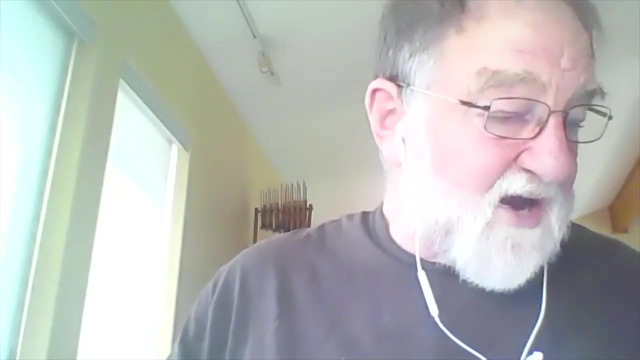 Yeah, that'd be awesome. So cadmium, copper, molybdenum, lead, zinc Are found in Fertilizers in low amounts because plants do need some nutrients but I don't think they need lead. So irrigation water you can find cadmium and iron. 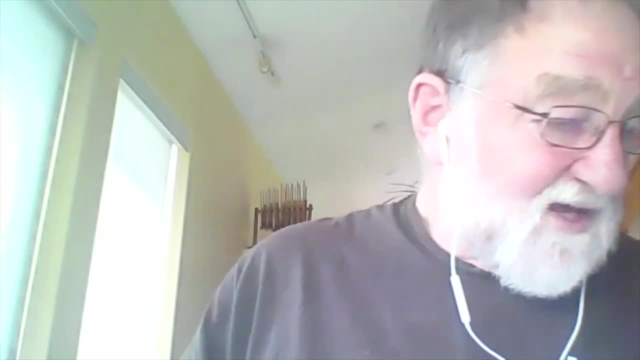 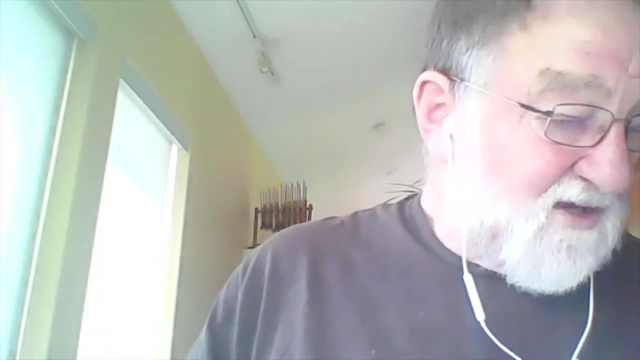 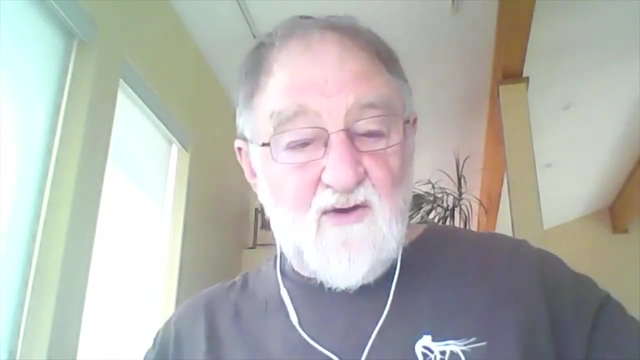 And iron is naturally high in the soils. anyways, Manures and compost. Here you get cadmium, chromium, copper, iron, mercury, manganese, molybdenum, Nickel, lead and zinc. all of those in high concentrations are going to be. 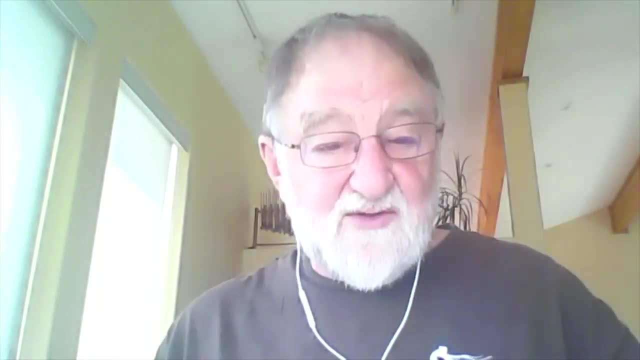 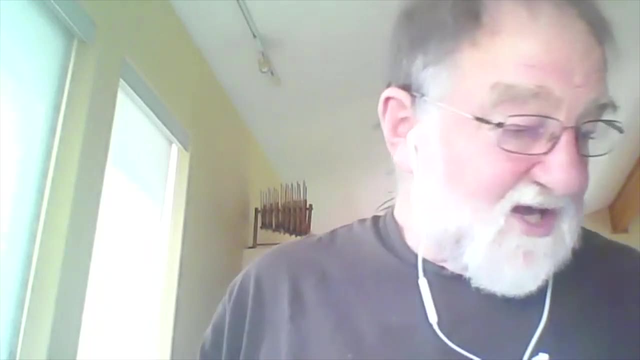 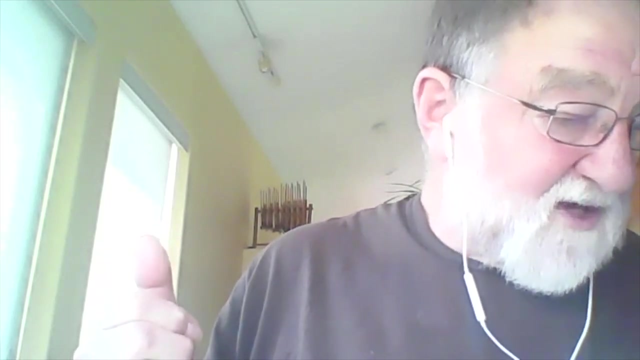 So if you're adding manures and composts, that's something you might want to test for. So, biosolids, this is interesting because you've got cadmium, chromium, copper, iron, mercury, manganese, molybdenum, nickel, lead zinc, copper, manganese again. 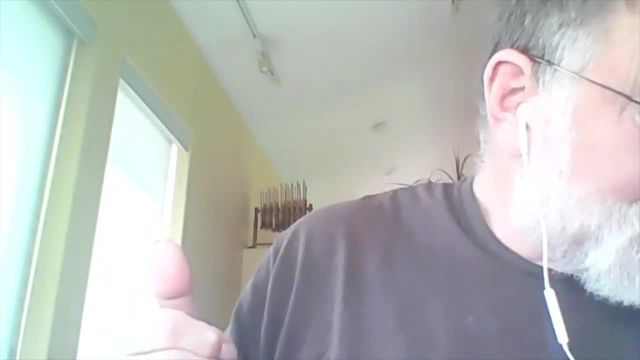 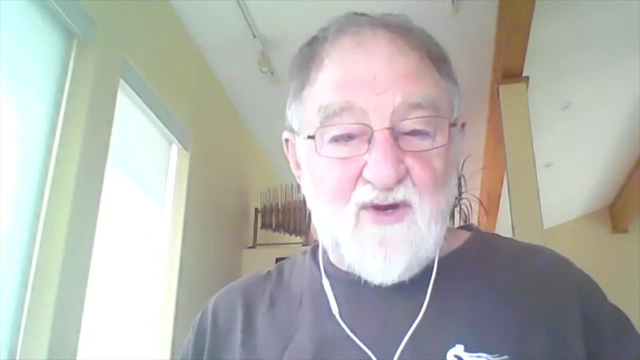 Oh, that's soil, sediments. Okay, Lead and zinc. So the biosolid industry. they're promoting using it, but they have concentrations of heavy metals And I don't know if they've got a way to remove them. Where are they coming from? 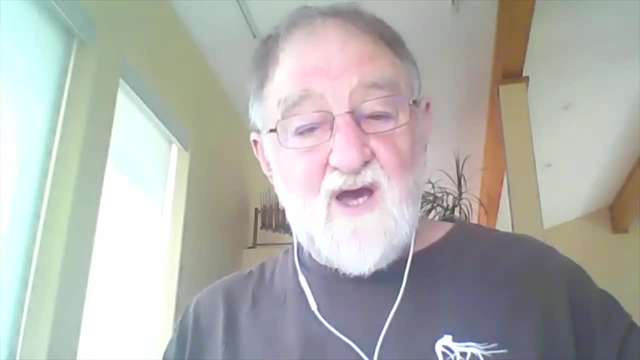 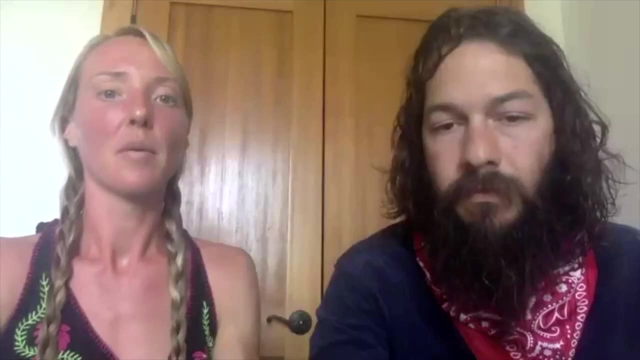 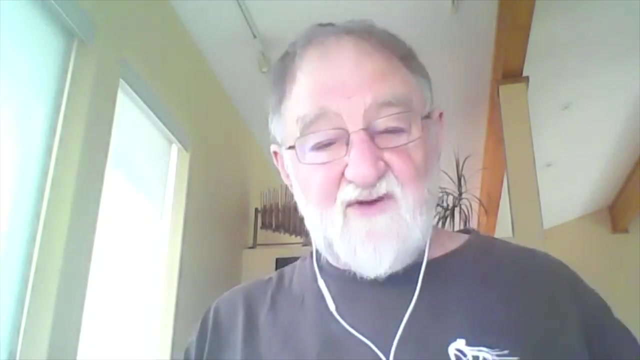 They're coming from. most of our cleaning products, birth control pills, everything that goes down the drain, Okay, Okay, So all of our household cleaning products. no idea what's in all of those things. That's where they're coming from. 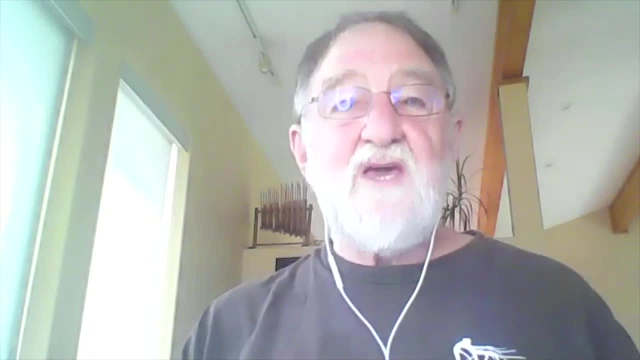 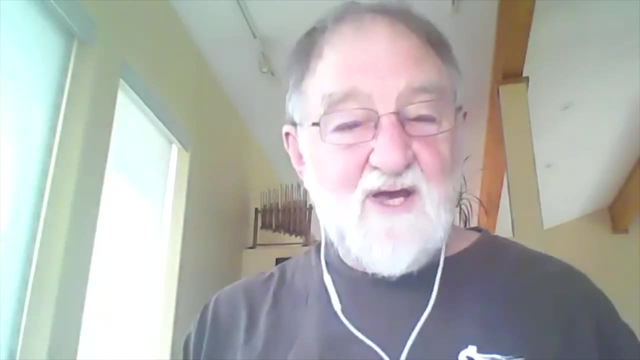 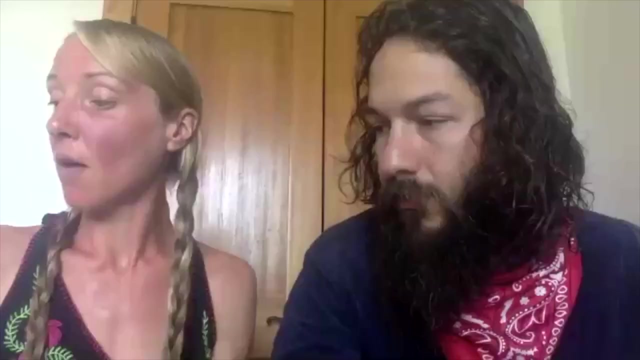 They're coming from the chemical industry. If we eat a normal diet and measure the heavy metals in our excrement, they'd probably be pretty low. It's all these other things that we put down the drain. Oh wow, So you are over on lead for animals. 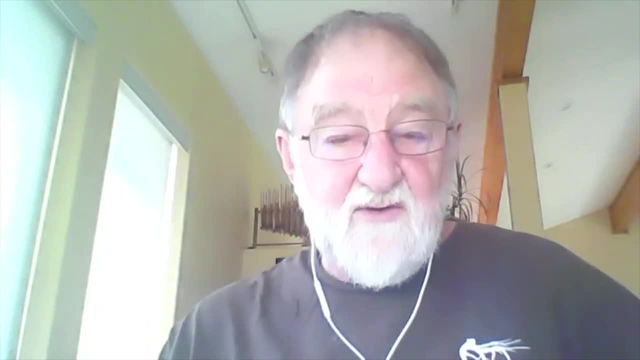 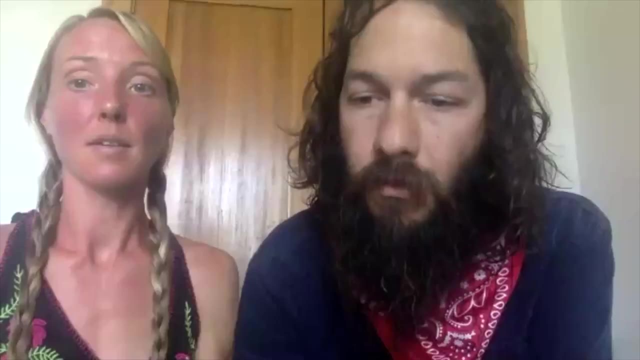 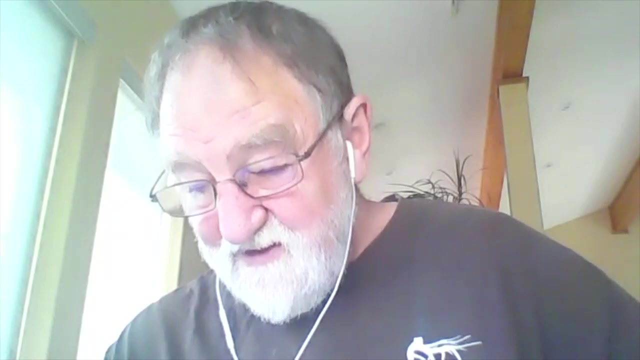 And that can be picked up, assimilated through plants. Okay, So that's the other thing you've got to look at is what elements are plants picking up Right? So the lead is high, And for industrial they're allowed 600 milligrams per kilogram. 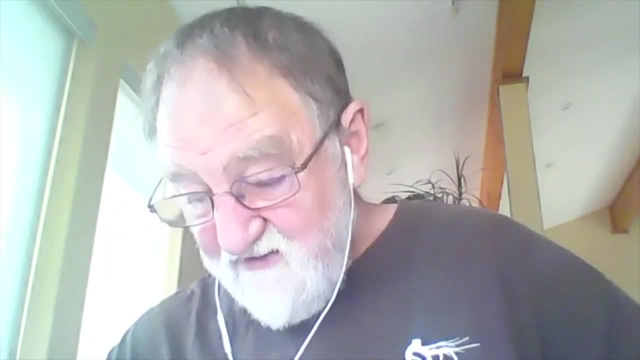 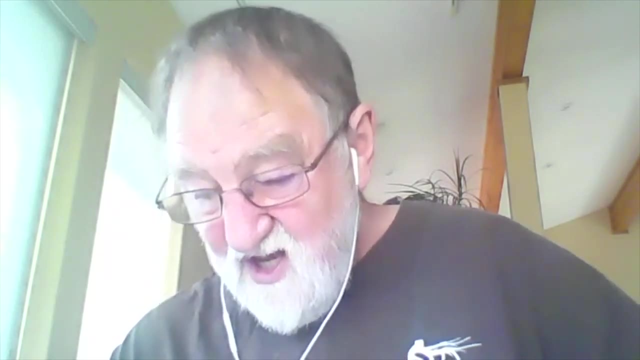 And then the zinc is 225 for you, The industrial is 410.. And 500 for cattle and horses. Wow, But the reason those two are high, when you look at your other numbers, they're all less than 20.. Right. 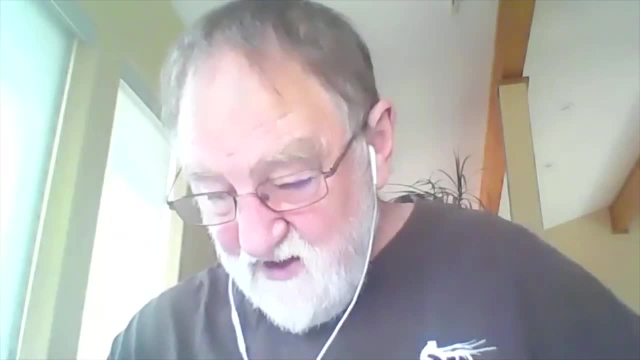 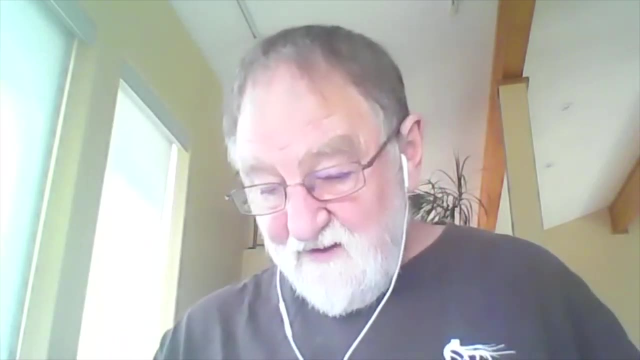 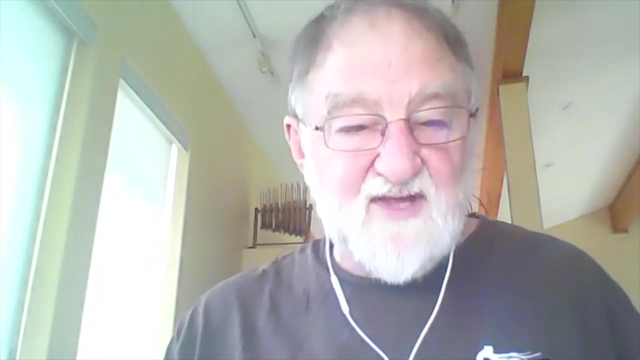 So those two are high because of the Kaminko mining operations that took place And the- you know, the tailings and from the air and all of that stuff. So that's why those two numbers are high, but they're still within the guidelines. 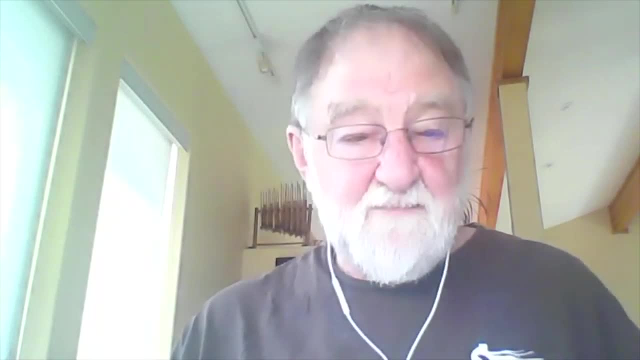 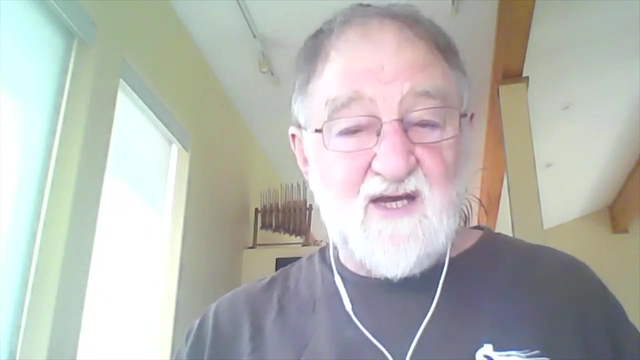 except for lead for cattle and horses. Right, Okay, So we have to do maybe more research. Oh, I did work for Kaminko back in 1972 and 73 in the Yukon prospecting as a student And we were always sending samples back and getting the concentrations of lead and zinc in those samples. 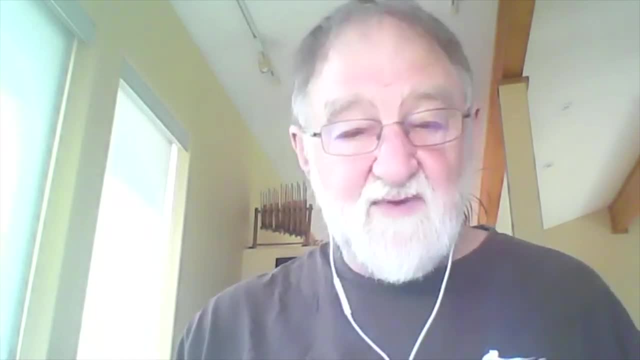 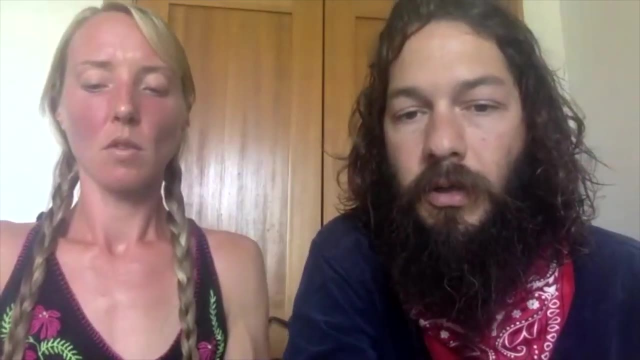 And they would come back pretty quick And they were pretty accurate as far as I know. Okay, That's good to know. Do you recommend that you know if people are leasing, if farmers are leasing land or they're looking at purchasing land? 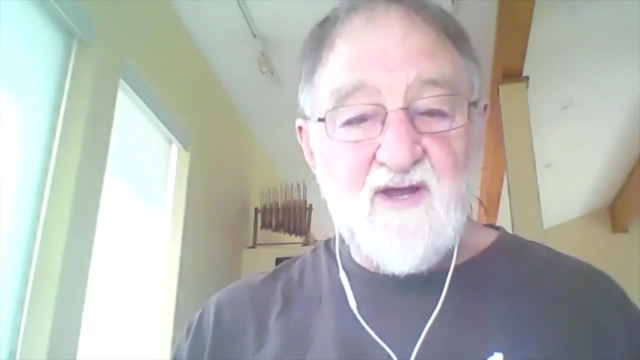 do you recommend doing heavy metal testing? I would definitely. If it's already a farm, you have no idea, right, Right, So I would do that. I would definitely do that before you made that purchase or lease it. Yeah, Okay. 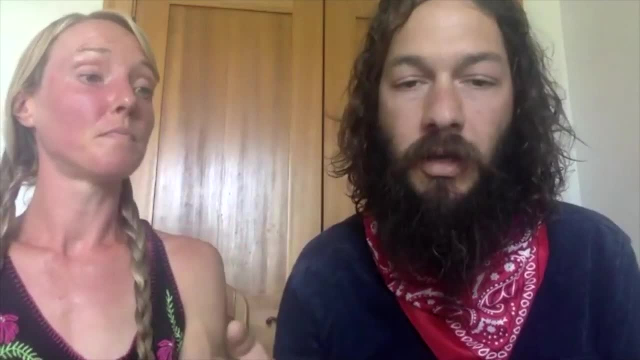 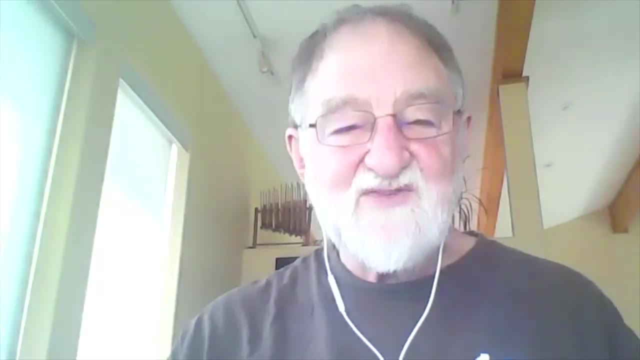 And we didn't know at the beginning either. We assumed that if we do a soil test, automatically they're going to look into heavy metals, But I guess that's not typical, right? Oh yeah, So you have to ask. No, you have to ask for what you want. Okay, You have to be very specific. Yeah, Because each one's a different test And, like you said, they're expensive. So, if you want to know what your nitrogen is, if you want to know what your phosphorus is, if you want to know those nutrients, you ask for those. 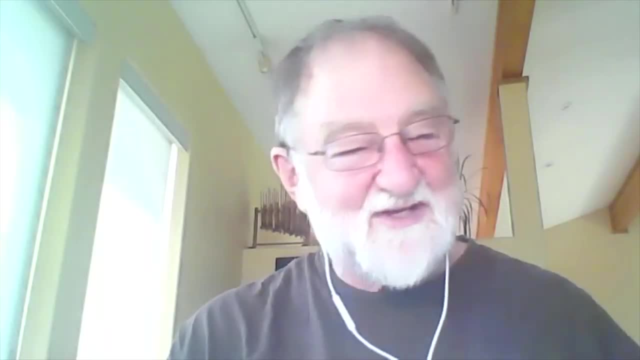 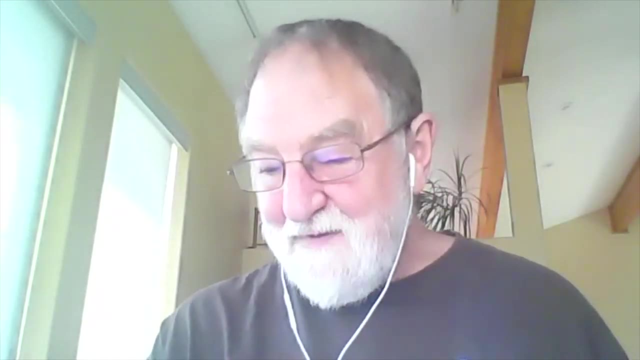 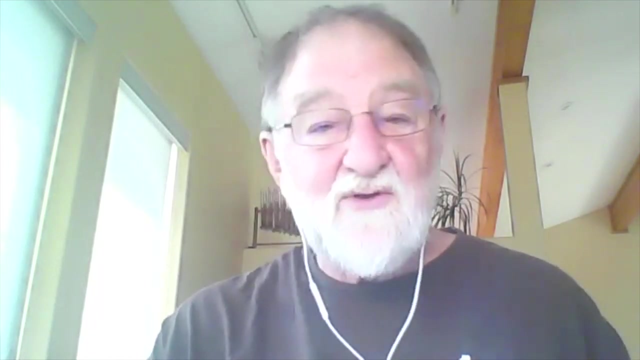 Yeah, Because I have this encyclopedia on soils- I mean, it's 2,000 pages, right- And I just looked up heavy metals last night and came up with this And it's a really interesting topic And I think, and also well, in the Arctic, I mean heavy metals are being carried in the atmosphere too, right. 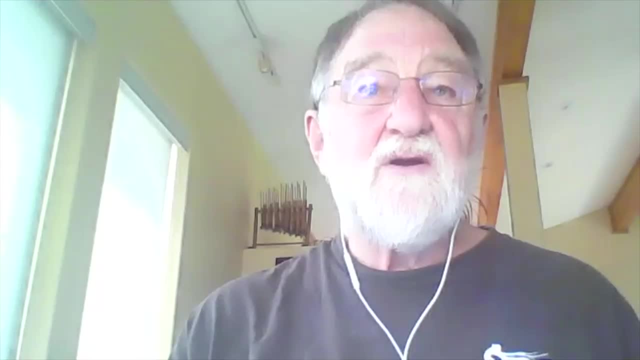 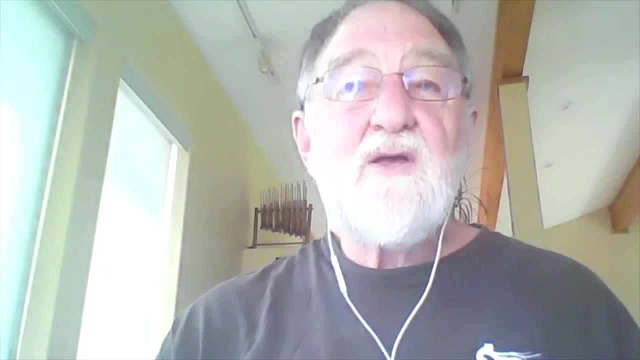 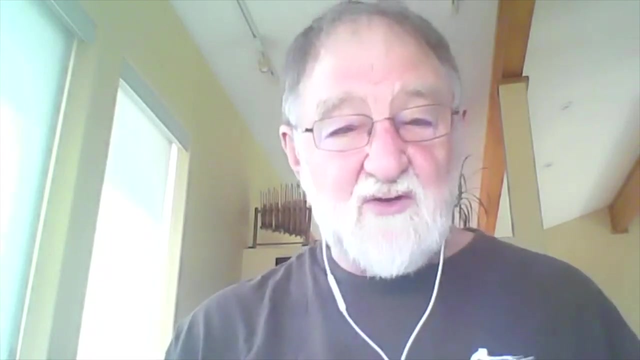 Right, You look at all the smokestacks. For example, here in Kamloops when Afton Mines was running, they had a smelter And they had a limit of pounds. They had a limit of pounds per mercury per day that they could put into the atmosphere. 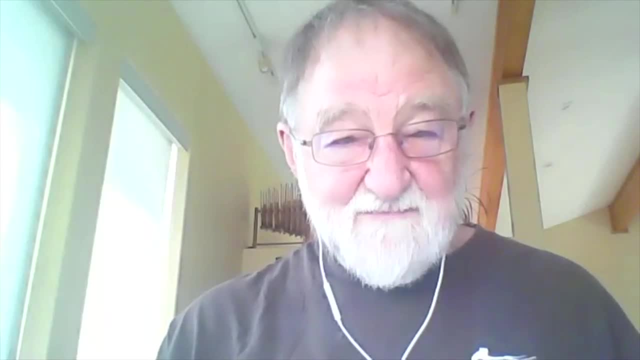 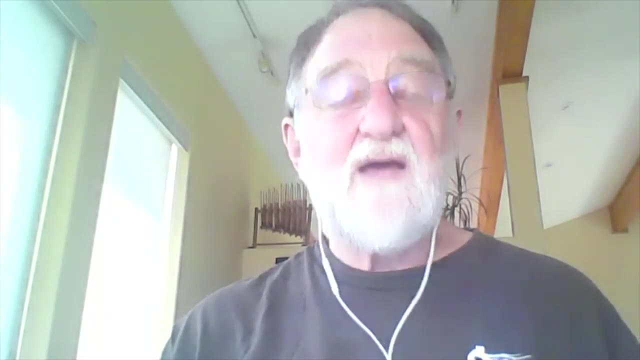 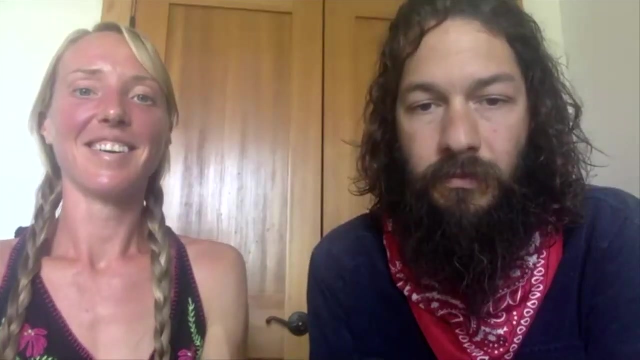 Every soil report that I saw of that because I was involved with the KPMG HMG Ajax review. Thank God that didn't go through. I'm going to be political here, So I reviewed the mercury level results from Afton Mines. 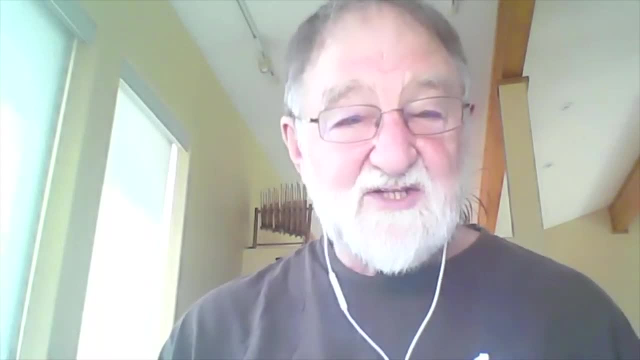 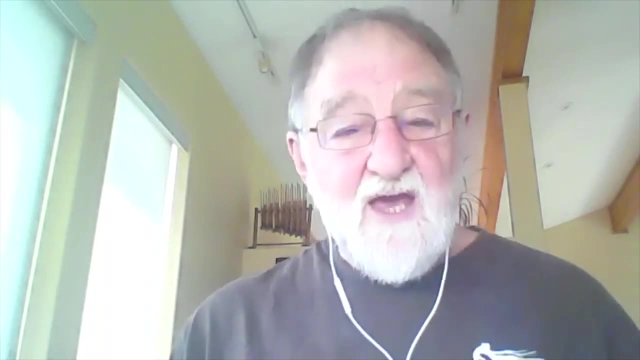 And they were always. and these were Environmental Protection Agency results Or no, the mine had to do the results. They went to the Environmental Protection Agency And in every case they were emitting 10 pounds of mercury a day. It was part of the smelting process. 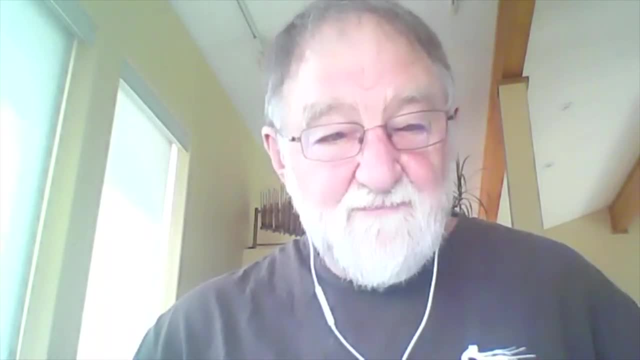 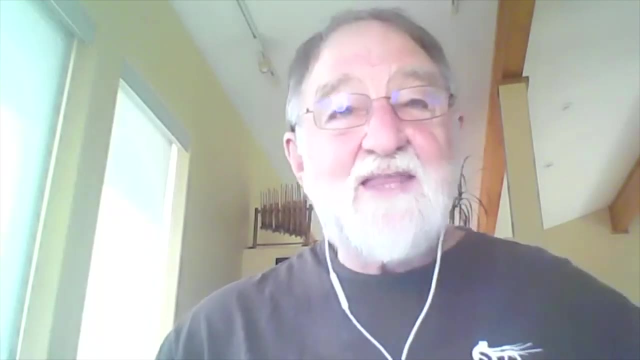 And the environment did not shut them down And that went on for, I think, three years. The concentration of mercury ended up just on the surface, just on the north end of the Overlander Bridge, Really In a trailer park there. 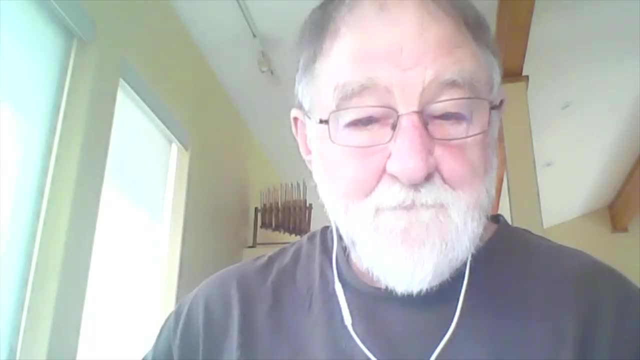 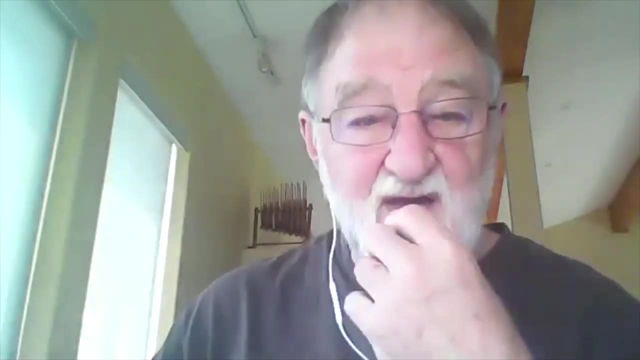 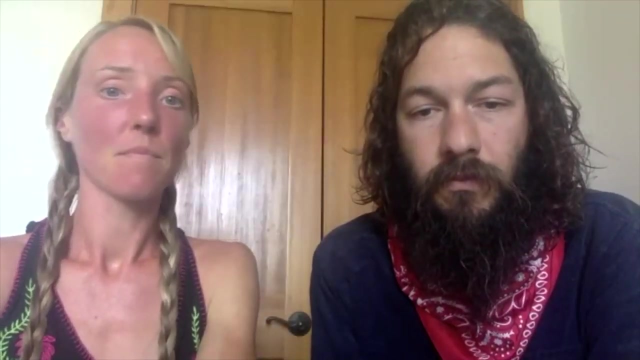 where the highest concentrations in the soil? Huh, Holy smokes. So the smelting process. that's why you have these high levels And Kimiko had all of this. Same thing happened in Sudbury, Ontario. That was a huge, huge area. 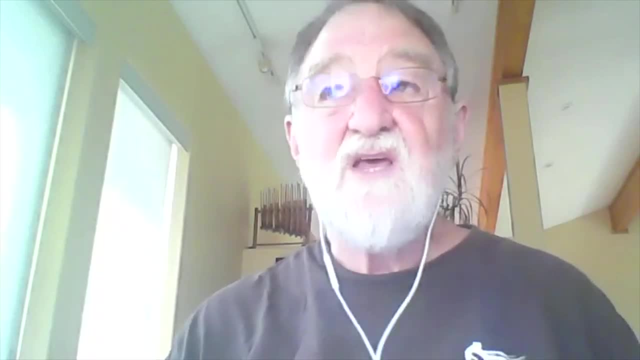 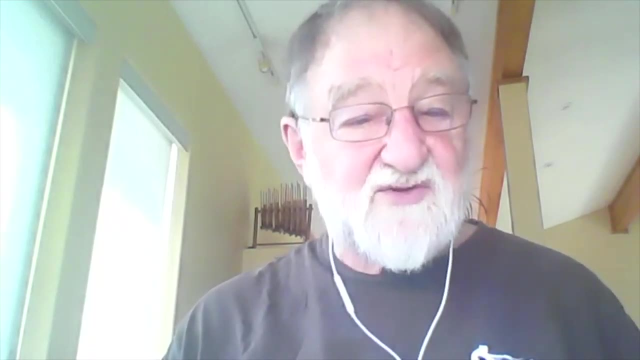 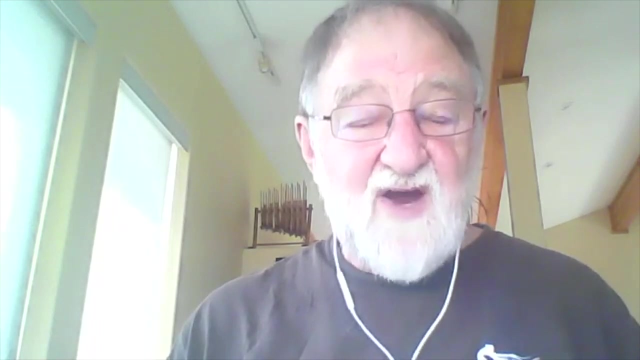 When I started doing remote sensing work back in the 70s. looking at the new satellite imagery we're starting we're starting to get in. the devastation from these smelters is horrendous, So it's carried in the atmosphere. They're finding higher and higher levels of heavy metals in the Arctic. 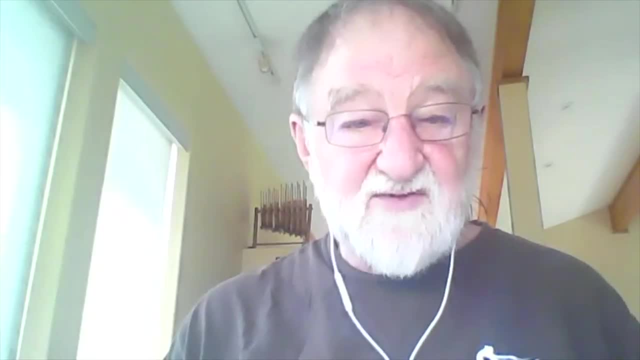 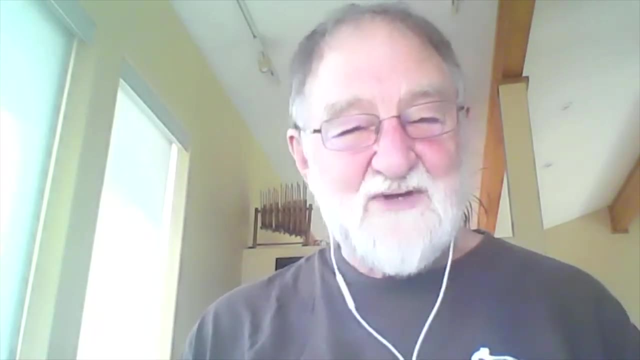 And that's going to be detrimental to wildlife. And so it's. it's in the atmosphere, It's it's: the more pollution we put out there, the worse it's going to get. Did you have my soils- textbook soils- illustrated when you took this? 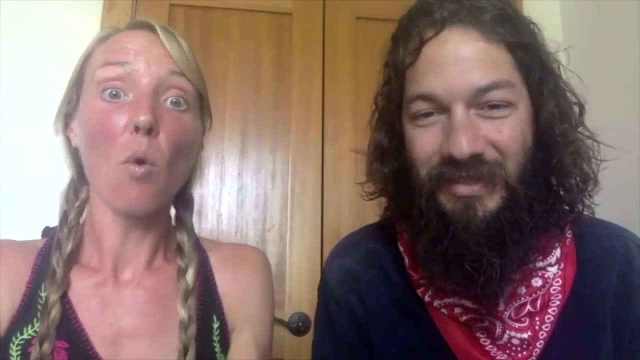 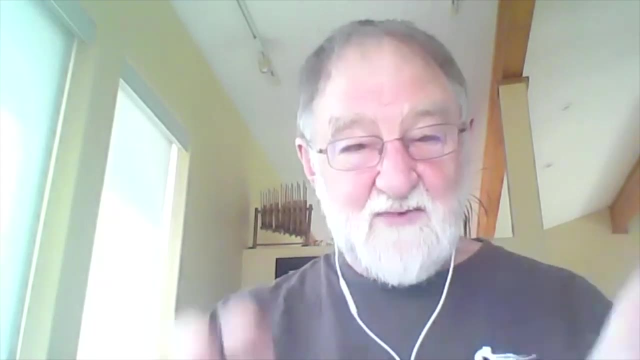 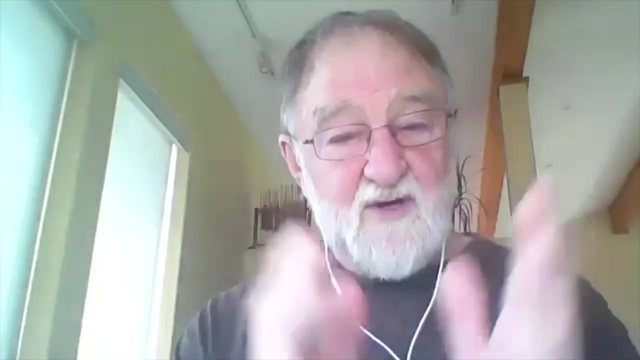 Yeah, Okay. So I'm planning a rewrite of that this winter. I have more, more photographs be more information, And I'm also, at the same time, creating a version for the onsite septic system people, because they just need- they don't need that whole book, but they need a condensed version. 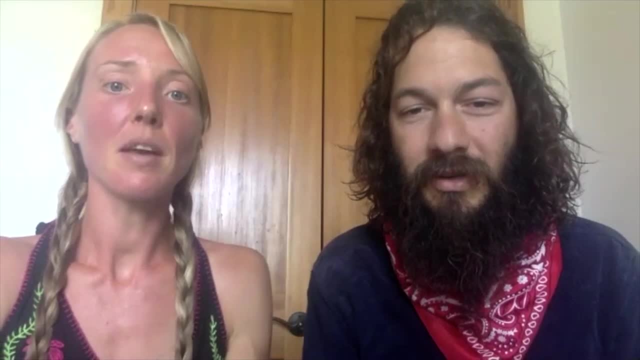 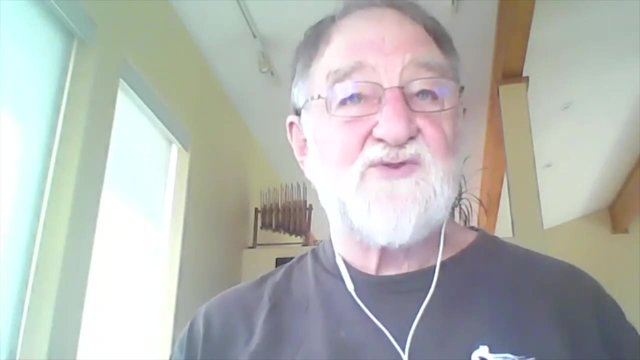 of it. So will it be? is it going to be available? Could we order it online? Could we get it? Yeah, Yeah, Okay, Yeah, Right now you can order. I'm soils illustrated through my website, edwardkentwatsoncom. 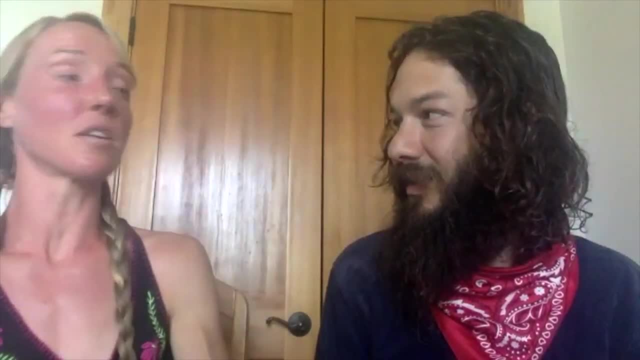 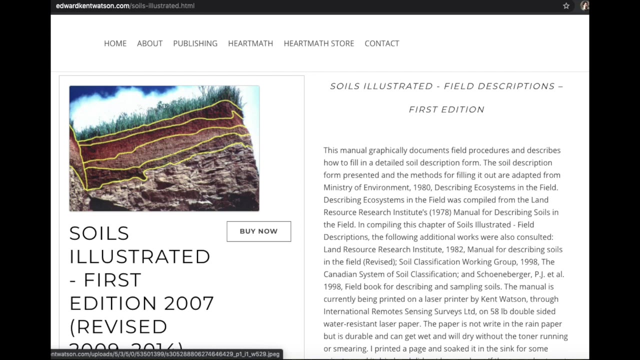 The soil. Well, the soils illustrated textbook is amazing. We still use it. It's the one of the very few books from university I kept with your soils illustrated, because it's again it's so clear. and the photos, the photos are amazing. That's what really helps when you're collecting soil for your sample to send away. It's best to get it from the top six inches of soil. You don't have to go that deep because most, most of them are in the top top bit of soil. 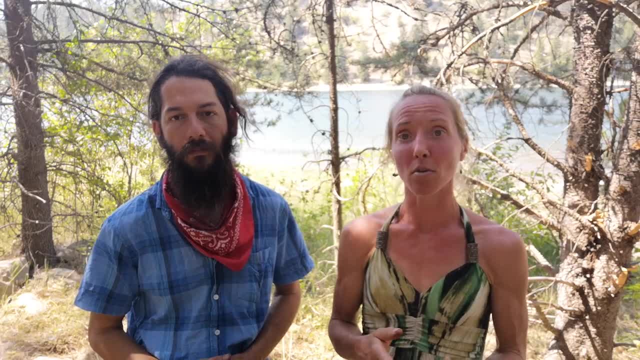 And then it's best to get it from the top six inches of soil, Soil, Soil. And then it's best to send it directly to a lab, not go through a middleman or anything like that. So find a lab that does the testing and send it to them directly. 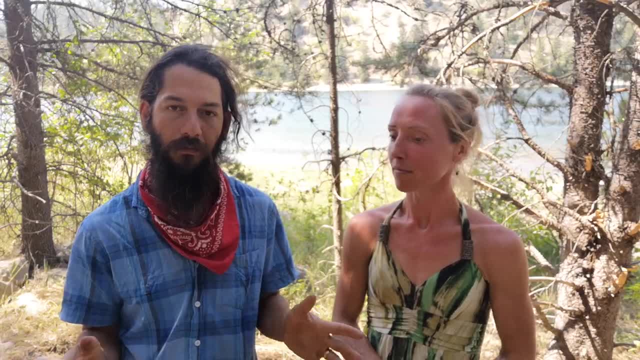 And it's very important to specify what you're looking for. There are generally two type of uh soil test. If, uh, you just ask for a sort of and don't specify it, they're just going to tell you about the fertility. 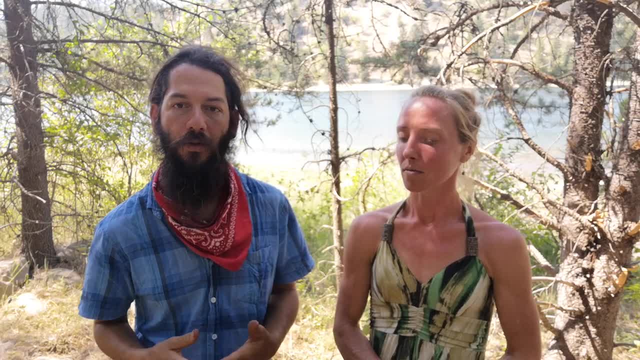 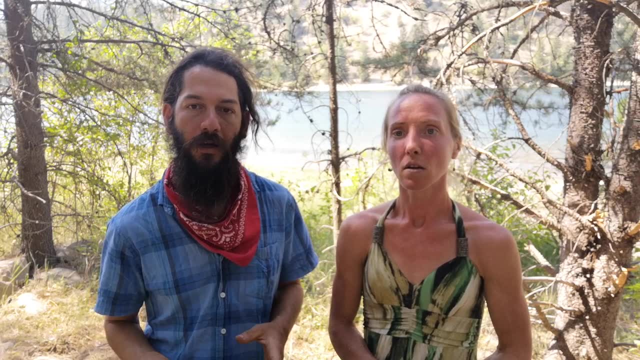 like the NPK levels and some other uh nutrients in the soil, But they won't tell you, like they're not going to test your soul for lead and mercury and our snake and things like that. So you want to specify. 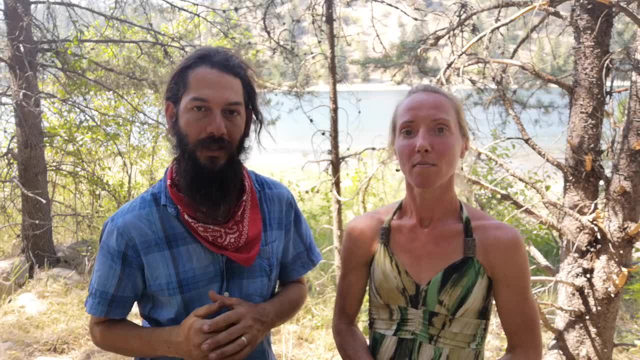 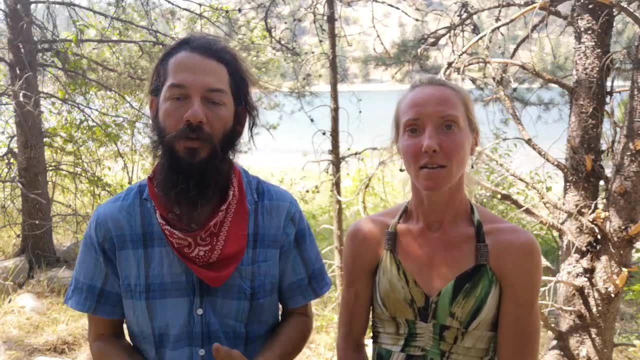 um, that you want to have all the different heavy metals tested and make that really clearly communicated with them so that you can get the right results back. now, when you get your soil results back, it's going to look something like this and you will see a table with a whole bunch. 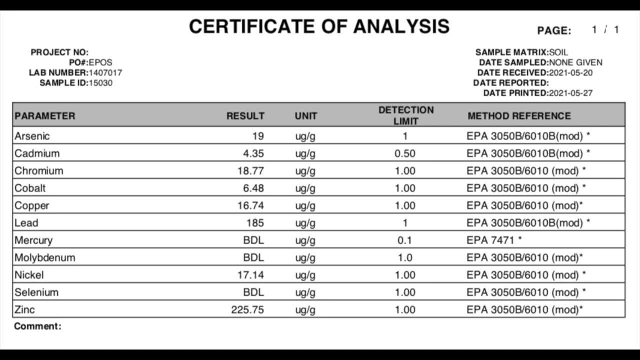 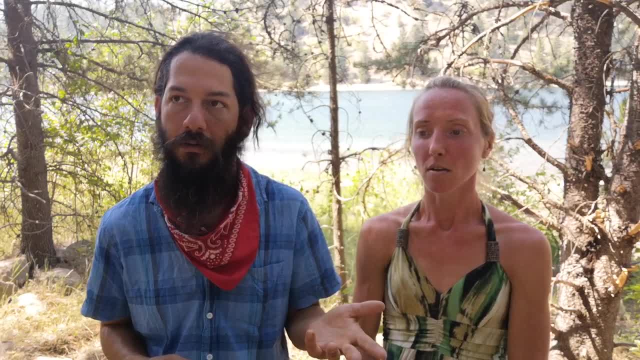 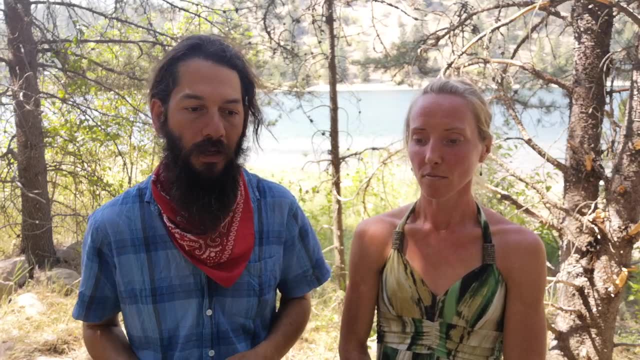 of different heavy metals listed and there will be the. the amount is going to be recorded in parts per million or micro, or milligram per kilogram or microgram per gram, and those units are all essentially the same. they're all parts per million and that's what the heavy metals are usually. 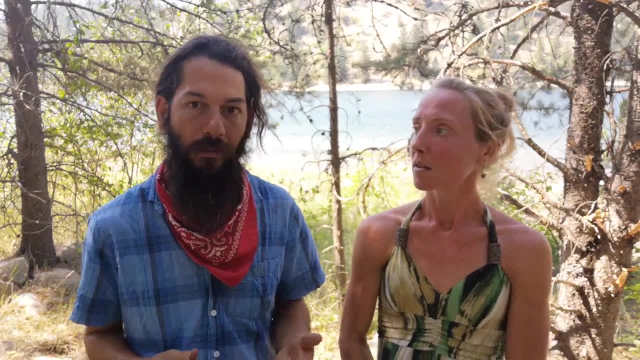 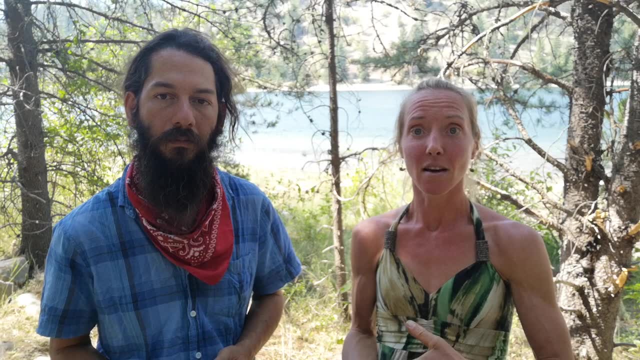 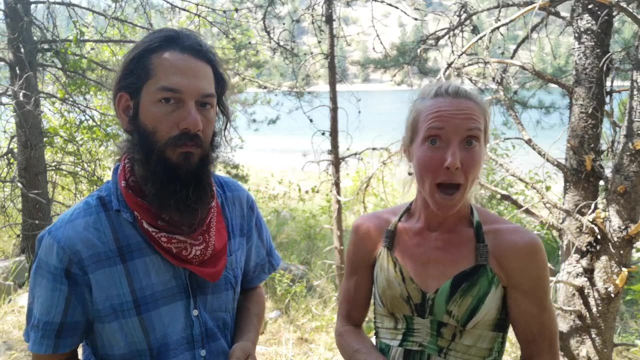 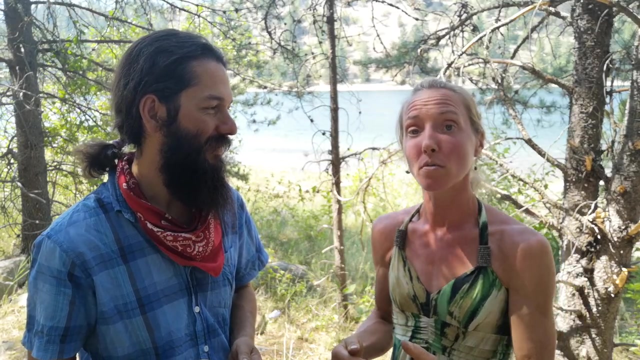 measured in in the soil and probably most of them are going to be present, right, yeah, yeah, because heavy metals occur naturally in nature, you will see some amount of- most likely, some amount of all the heavy metals present in your soil. so don't panic. now is the time to use your head, use your brain and do some research and compare your results to 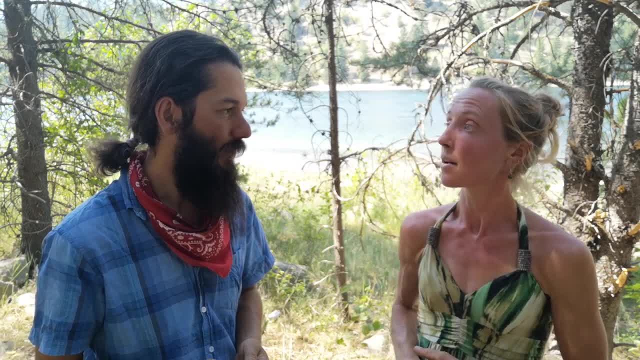 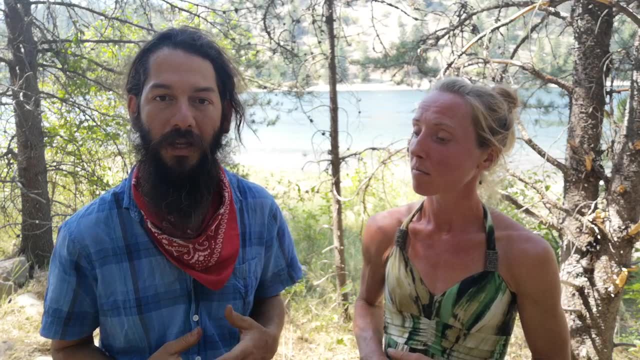 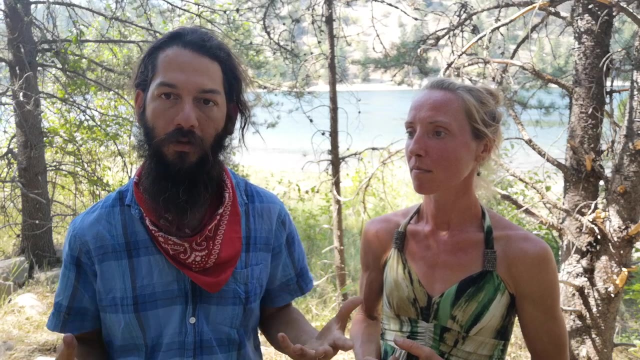 literature of safe levels. so yeah, and we started doing some literature review when we got our results and found a few references. but it's a pretty tedious process. so we were so happy to talk to Kent and he cleared a lot of things up and he did mention that you know our soil. 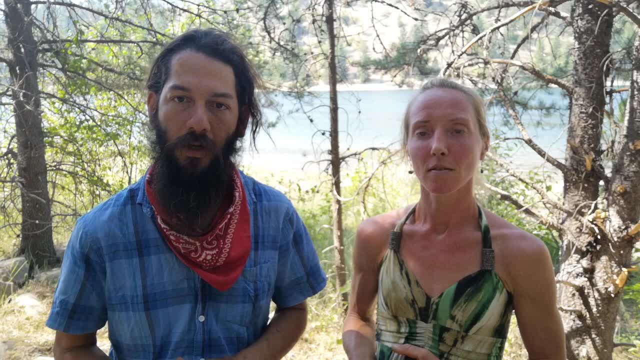 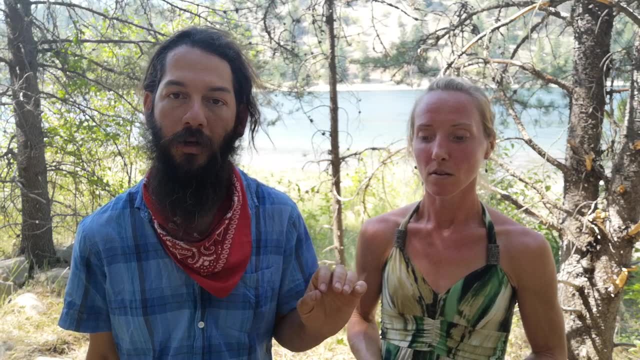 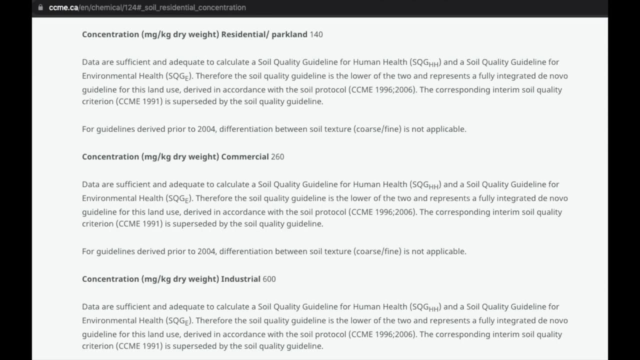 is safe to use. the only thing that stood out was the level of lead. so, uh, specifically, our soil has a little bit higher amount of lead than is set as a standard in Canada. so there's an organization that in Canadian organization in 1999 that I will put a reference in the video, that they provided health guidelines. 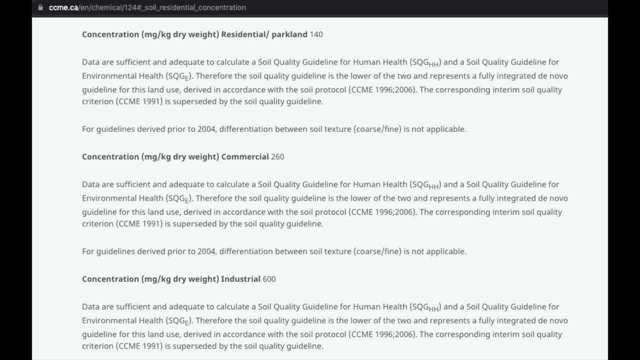 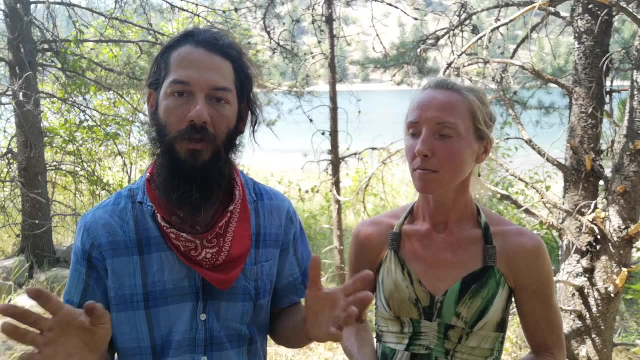 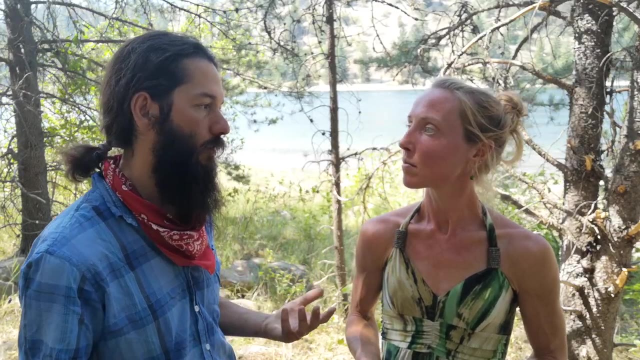 for amount of lead in soil and they said 140 parts per million is sort of like a natural safe guideline. now, different countries, different regions in the world, they have their own guidelines and they're all over the place, and so in many of those cases we actually fall within the safe region. but in Canada, um, our lead is a little high now. 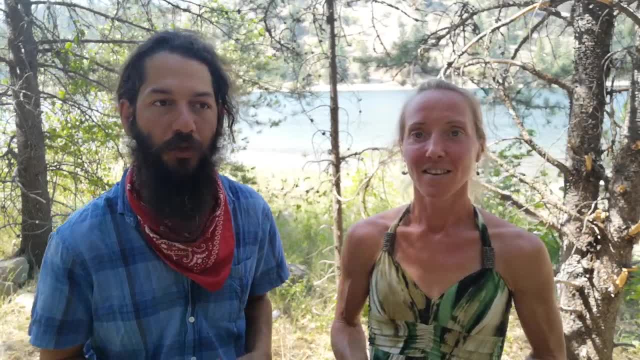 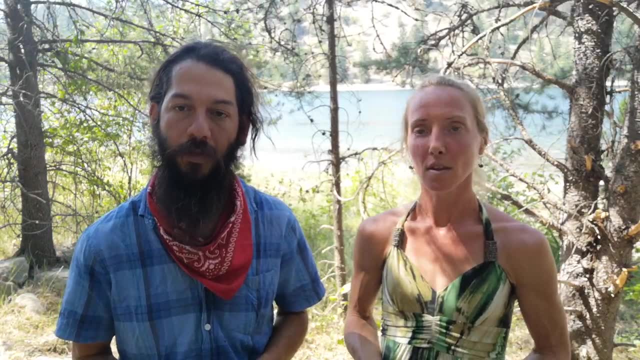 this doesn't mean that we just need to panic and run away. just we need to keep that in mind with how we are, uh, doing our agricultural work here, that there is a little bit of excess lead, and so we need to come up with strategies to deal with that or work around that. 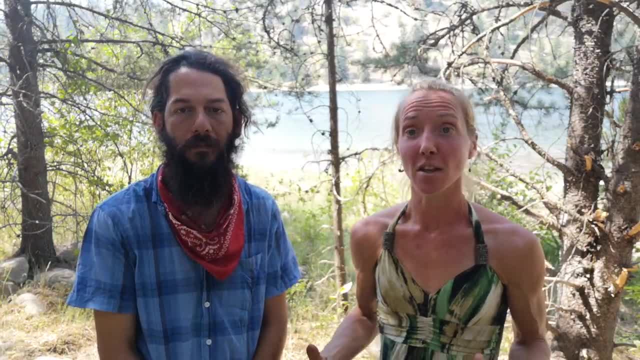 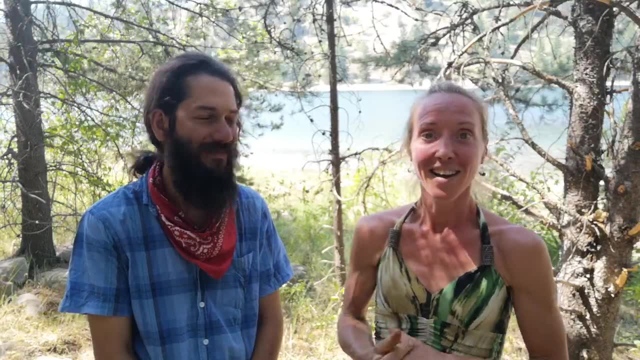 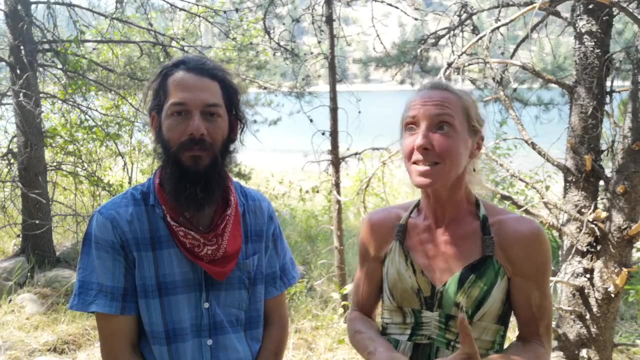 it. so what can we do to deal with this extra lead that's in our soil? well, there's a few different methods. one of them is phytoremediation, which we're very excited to try. it's the use of plants to capture the excess heavy metals in soil. so, for example, sunflowers- yay comfrey, they'll capture lead. 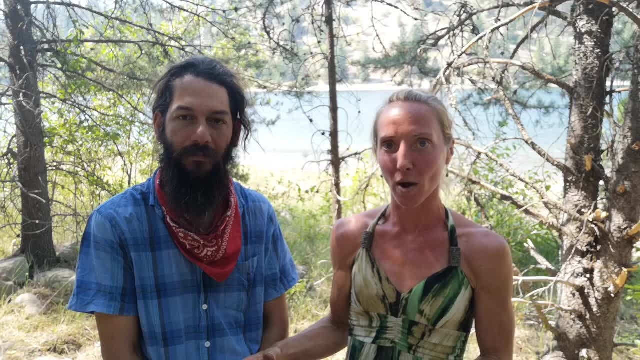 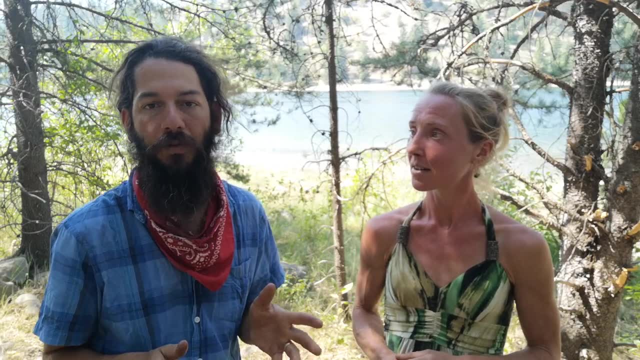 and then you remove the plants out of the soil and compost them in a certain way that so that they don't re-enter the environment. now, lead is one of those heavy metals. that is actually not a huge problem if you are growing fruit or berries, because the plants do a pretty good job of. 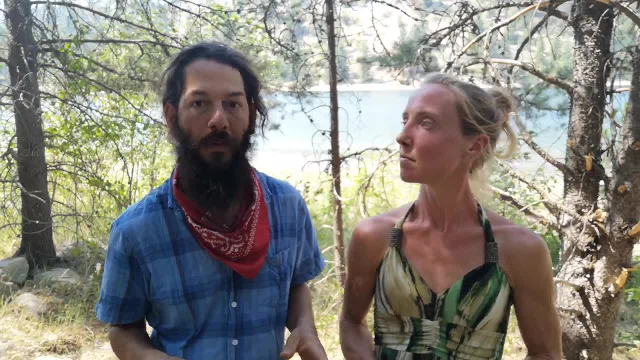 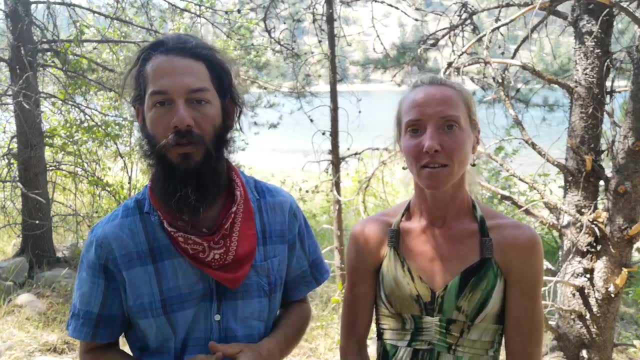 filtering that out. so that doesn't actually get you know. many people think that you don't know if your soil is contaminated. plants are gonna basically suck everything and it's gonna. you know all everything you grow is gonna be contaminated, but actually that's not the case. so there's many different filtering that happens in different plants and the way actually 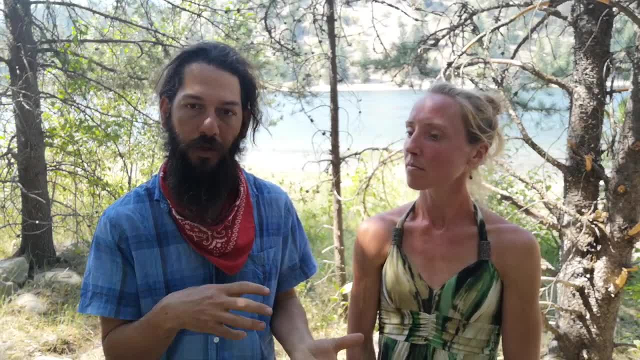 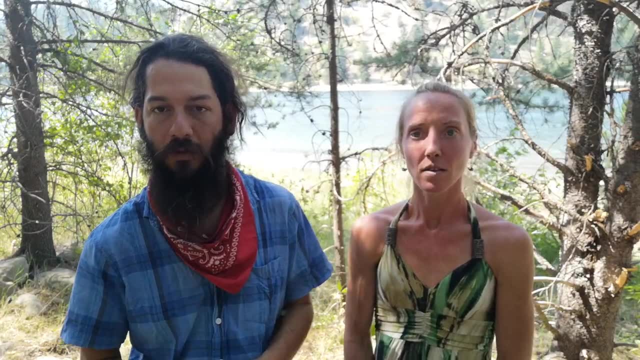 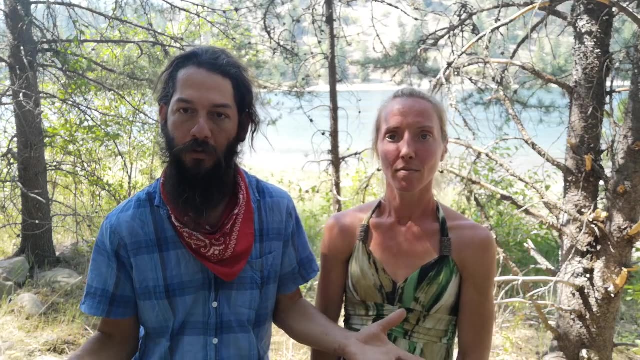 lead ends up in our system is usually not because it's getting sucked into the food, and vegetables is usually because dirt gets picked up and then gets connected to, for example, leafy greens and things like that. so we just have to be smart about how we plant, for example, our own garden, for you know, for the 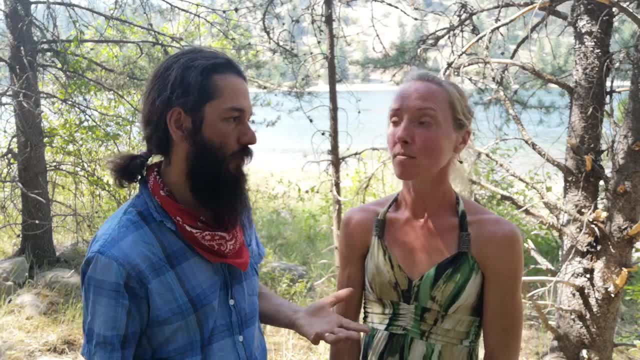 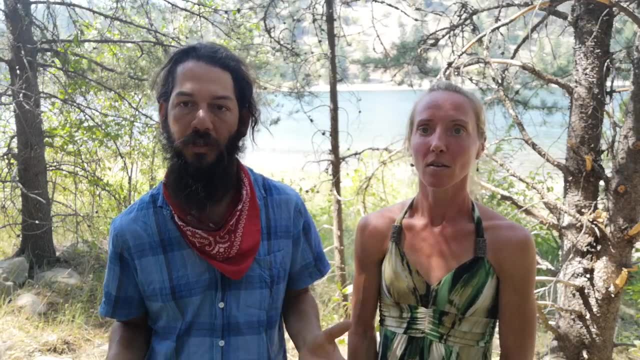 vegetables that we're growing for ourselves. but as far as our main plant, which is growing the orchard, it doesn't pose any threat because the trees are gonna do an, you know, amazing job. the berry bushes are gonna do an amazing job of filtering everything out. so we are gonna be good to go there. we're gonna continue doing. 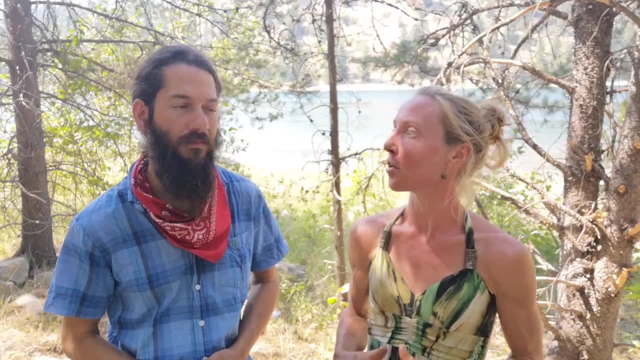 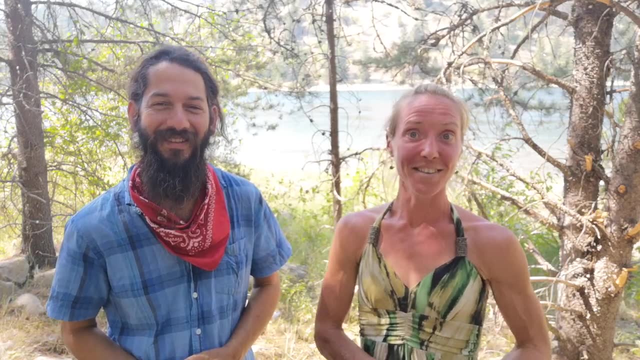 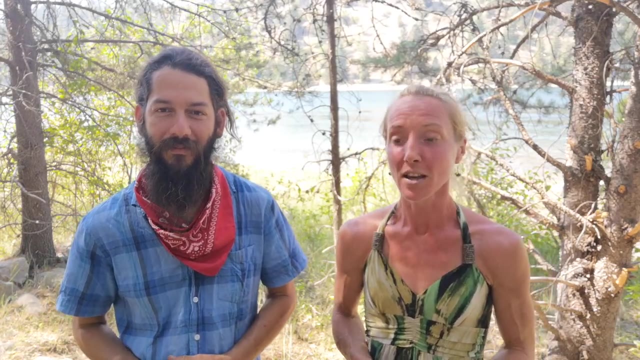 research, research on this topic, because it there is a lot to know in. yeah, and it's a heavy one. but we are also going to keep in contact with Kent Watson and hopefully have another interview with him in the future to learn a bit more about everything. so if you have any questions or 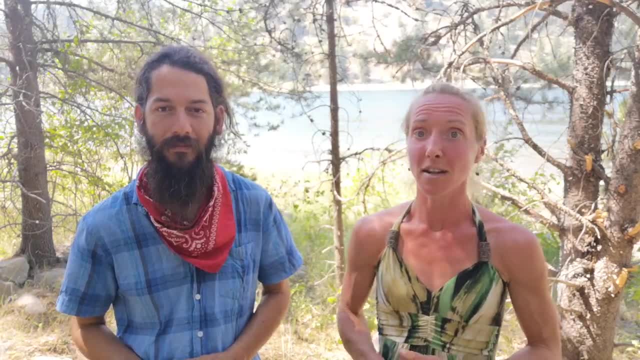 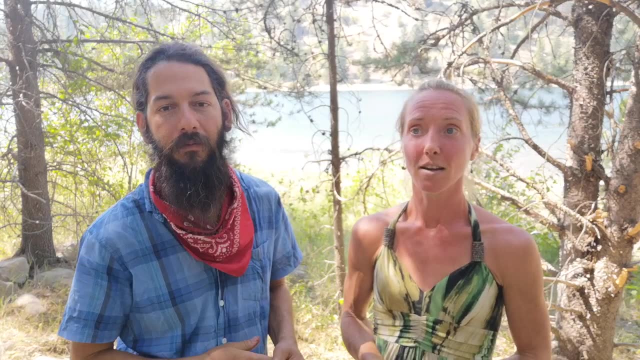 concerns or anything, please feel free get in touch with us and we can either pass them along with Kent or pass along any information that we might have. yeah, and actually, if you want to stay in touch and see our video videos, a lot of our friends actually miss our videos once in a while because it gets. 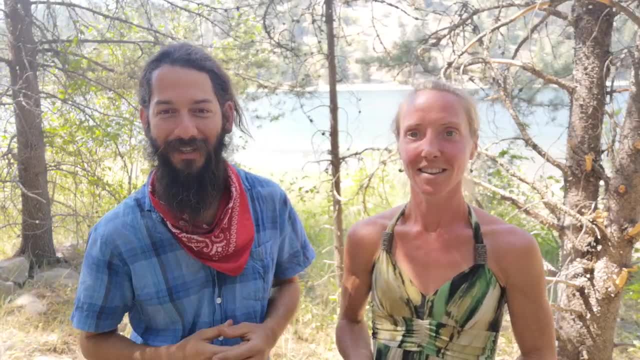 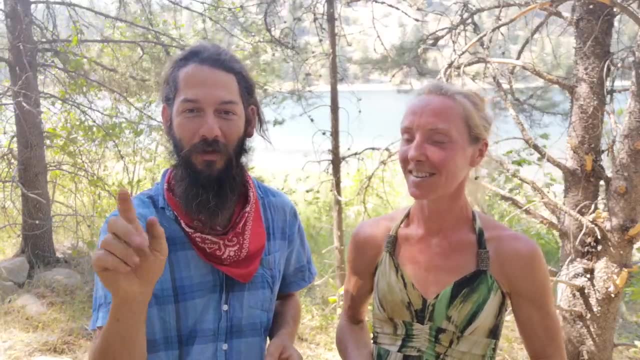 buried in? we still we don't have a. you know we don't get a lot of attention on YouTube. it's just a group of friends and family, basically, that are watching you right now. yeah, but if you want to stay in touch- one of the great ways to use the bell- and then if you hit that Bell, you get a. 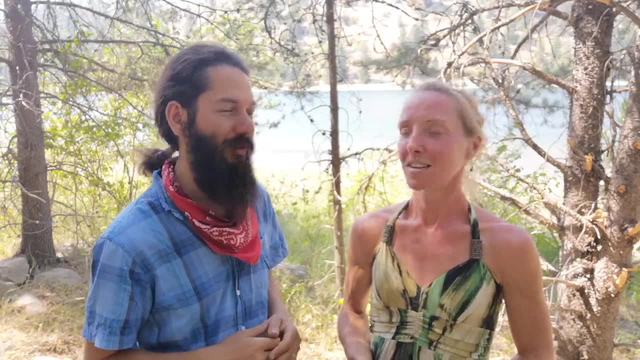 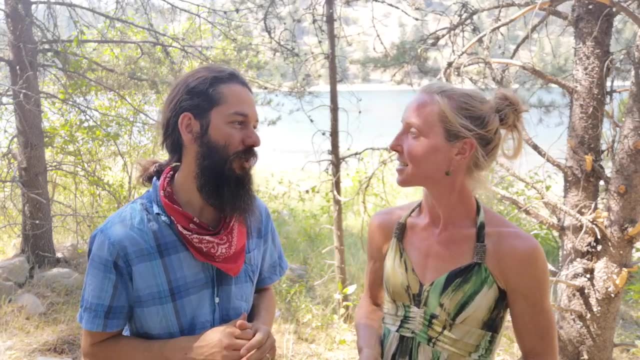 email every time you put a video out, which is every Sunday, hopefully, unless we're really late today, but you should still get it today and, um, yeah, just keep that's it, I think. just keep in touch, and we would love to hear comments and questions from you, and we will see you next week.